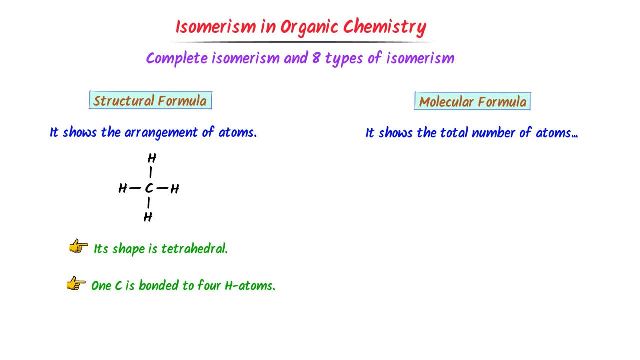 total number of atoms. For example, the molecular formula of methane is CH4. It shows that there is one atom of carbon and there are four atoms of hydrogen present In a single molecule of methane. Thus we learn that structure formula shows the arrangement of. 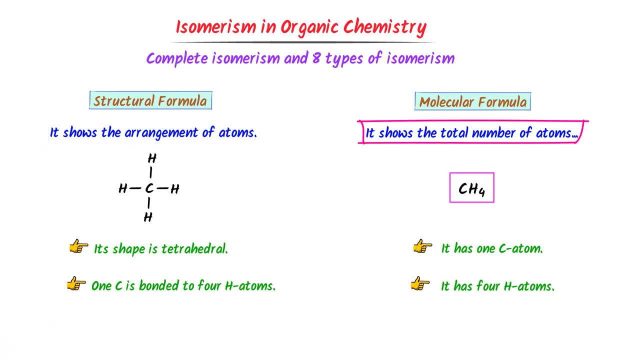 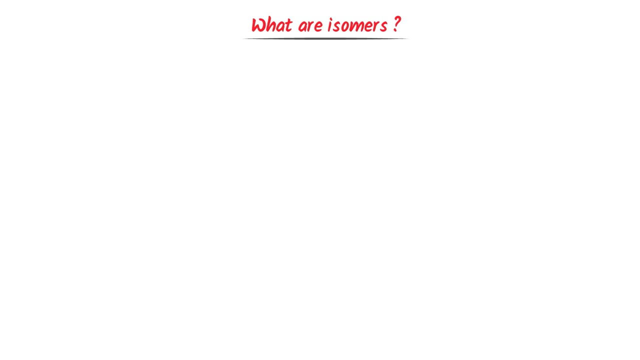 atoms in any compound, while molecular formula shows the total number of atoms present in a compound. Hence, noted down these fundamental concepts. Now, what are isomers? Well, I always teach this simple analogy: Consider these gloves. We know that this glove has four. 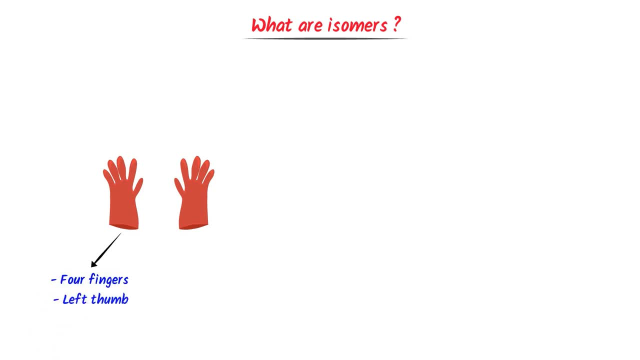 fingers and it has one left thumb, while this glove has also four fingers and it has one right thumb. I say, both gloves have four fingers and a thumb, but they have different arrangement. Now listen carefully. Gloves are isomers of each other because they have same number of fingers and 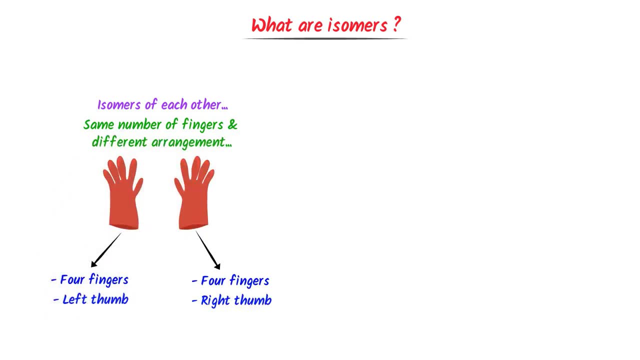 different arrangement. Let me repeat it: Gloves are isomers of each other because they have same number of fingers and different arrangement. So the easy trick to remember the concept of isomer is: they must have same number of fingers but different arrangement. Now consider these. 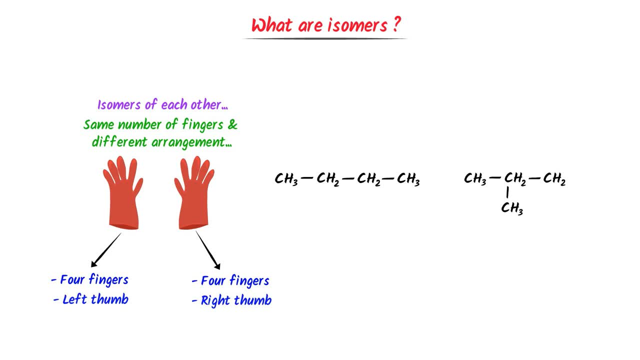 organic compounds. Let me find the molecular formula of this compound. We can see that there are four carbon atoms present in it, while there are ten hydrogen atoms present in it. So the IUPAC name of this compound is n-butane. On the other hand, there are also four carbon atoms. 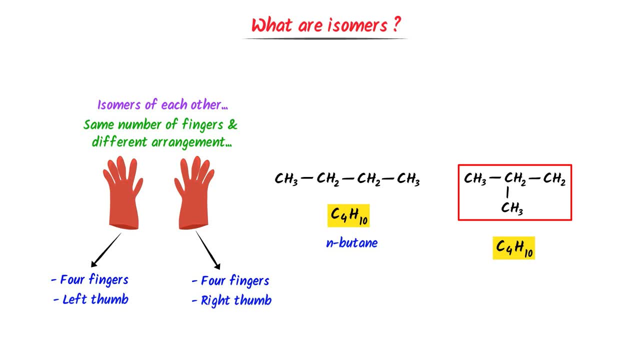 present in it, while there are also ten hydrogen atoms present in it. Here I write 1,, 2,, 3.. The methyl CH4 is bonded at the second compound. Now let me write 1,, 2,, 3.. The methyl CH4 is bonded at the second. 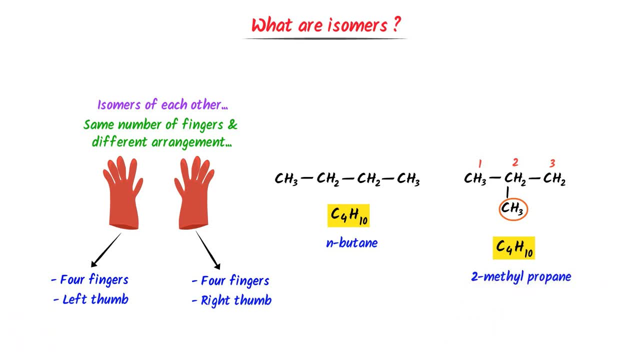 carbon. I write 2-methyl propene. Now listen carefully. This compound and this compound have the same molecular formula- C4H10, but different arrangement, So they are isomers of each other. Let me repeat it: This compound and this compound have the same molecular formula, C4H10,. 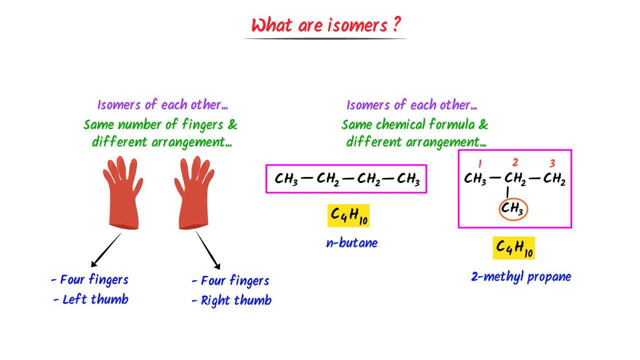 but different arrangement. So they are isomers of each other, of each other. Thus, remember that these both compounds have same fingers or molecular formula, but they have different structure, formula or different arrangement. Therefore, we define isomers as the chemical compounds which have the same chemical formula but different structure. 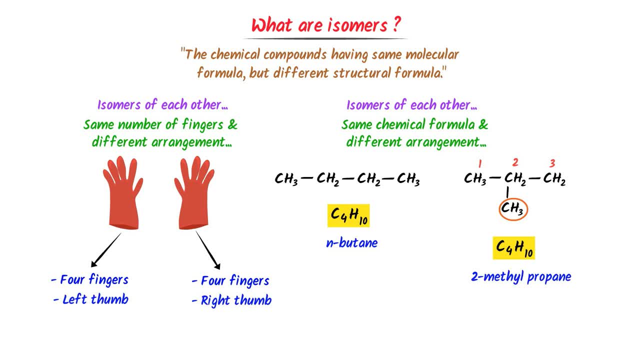 formula are called isomers. For example, n-butane and 2-methylpropane are isomers of each other because they have same molecular formula but different structure or different arrangement. Thus note it down, this easy concept of isomers. Here let me ask you one of my favorite questions. 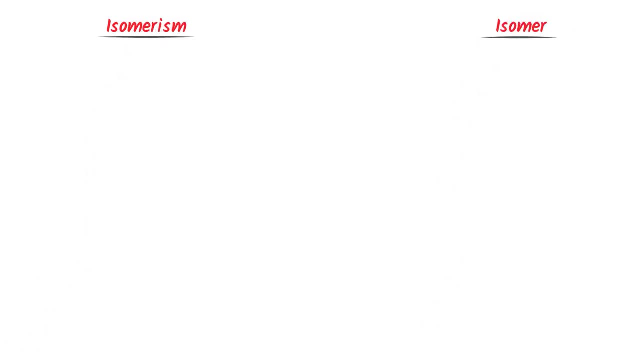 What is the difference between isomerism and isomers? Well, believe me, many students know its definition, but they do not know its concept. Let consider hands and a nose. I say isomerism is possible in hands because we have one left hand and 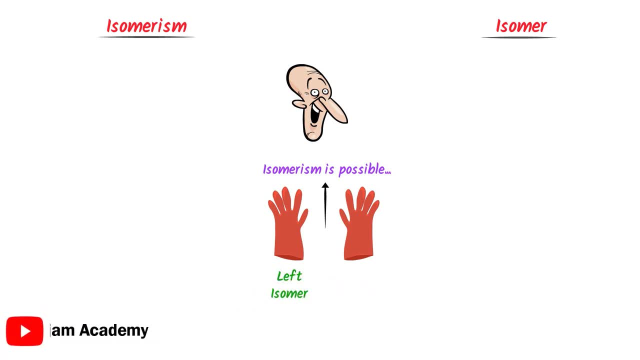 one right hand or one left isomer and one right isomer. Secondly, I say that isomerism is not possible in a nose, Because we have only one nose. It has no other isomer. Therefore, personally, I say that isomers 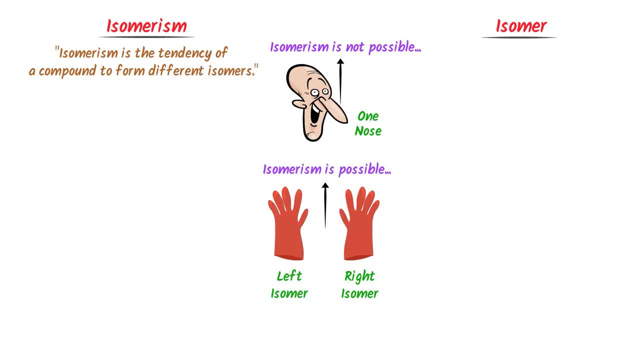 is the tendency, ability of any compound to form different compounds having different structures. For example, our hands have the tendency to form two compounds having different structure, while isomers are the outputs of isomerism. Things being some know, asnes and the familiae are different cell type. 너무 여 astronomical. 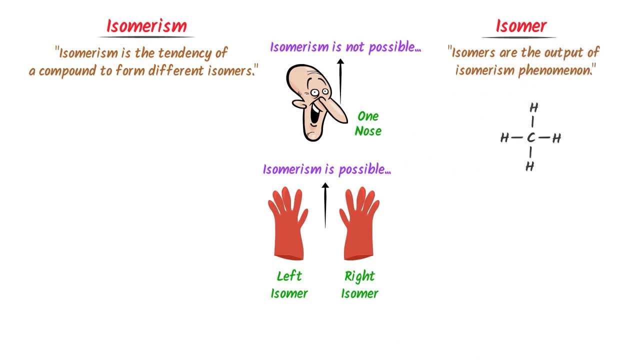 accommodation where the planets didn't add, though, we have floating isomers being whole, you powder which stabilized the real 1986, if you previously answer bye to cans or Weed, For example, consider CH4. We say that isomerism is not possible in CH4, so it has no isomer. 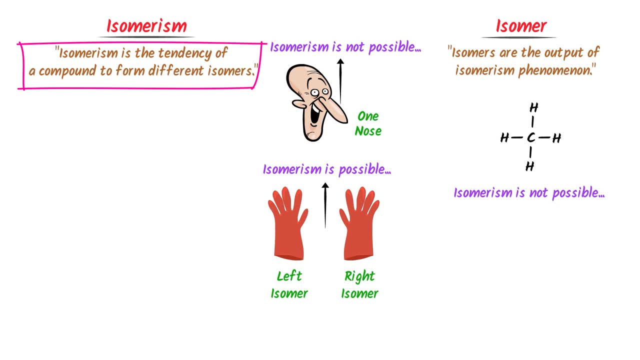 Thus, remember that isomerism is the phenomena or tendency of a compound to form different compounds having different structures, while isomers are the output of the isomerism. Here remember this bonus point: Isomers have different physical properties. For example, consider these two isomers: This is alcohol and this is ether. We know that they have. 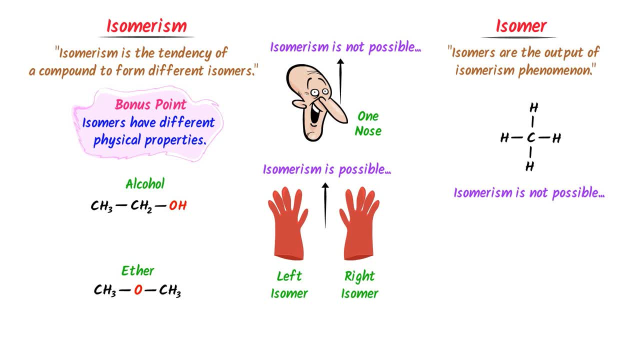 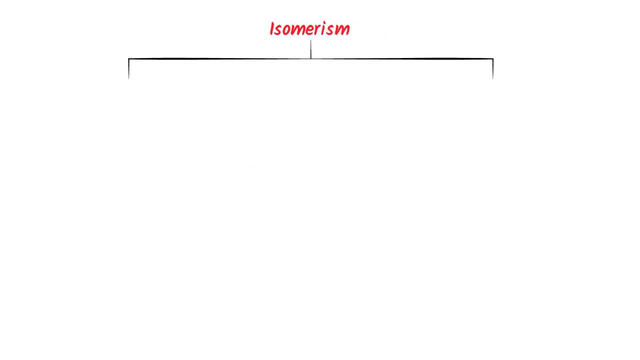 same molecular formula, but they have different structures. That's why they have different physical properties. For instance, this is liquid and this is a gas. Therefore, we say that isomers have different physical properties. Now we will learn the type of isomerism. Well, there are two types of isomerism – structural. 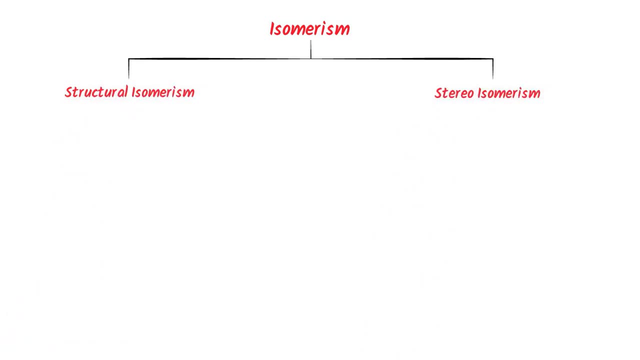 isomerism and stereo isomerism. Structural isomerism is further divided into six categories like chain isomerism, position isomerism, functional group isomerism, metamerism, tautomerism and ring-chain isomerism. 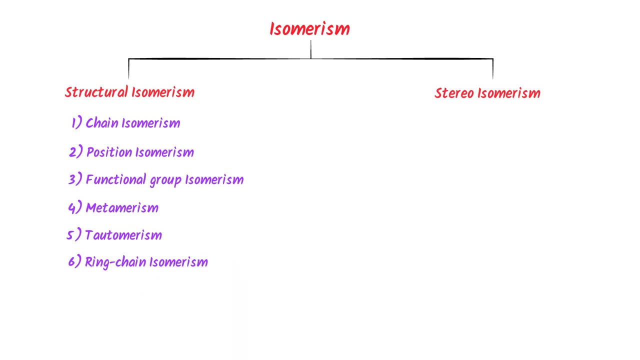 Here are some examples of chain isomerism, While stereo isomerism is further divided into two categories: geometric isomerism and optical isomerism. Hence, these are the eight different types of isomerism. Now we will learn chain isomerism and position isomerism. 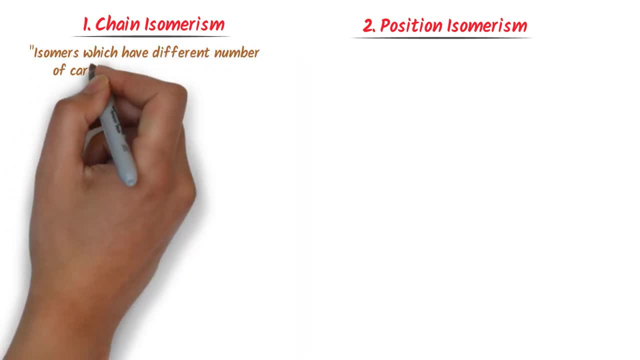 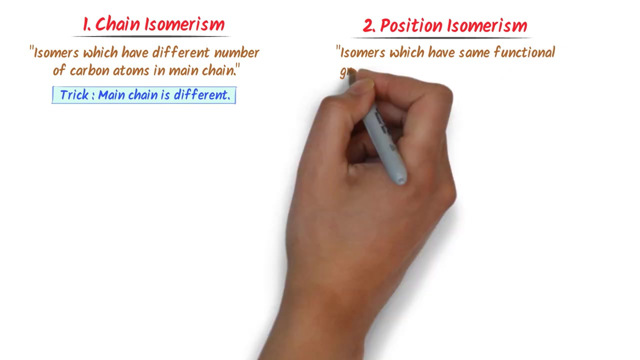 Well, those isomers which have different number of carbons in main chain are called chain isomers. The easy trick is: the main chain or the parent chain of carbon must be different, while those isomers which have same functional group attached at different position are called position. 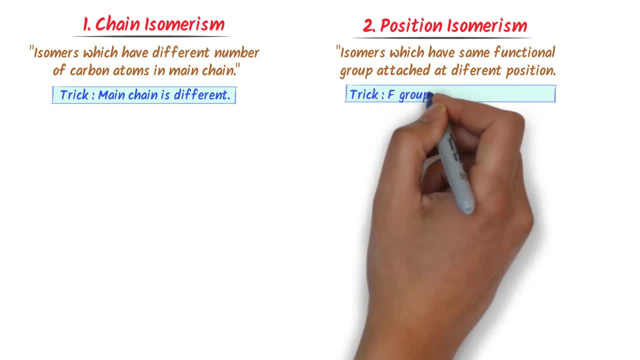 isomers. The easy trick is functional group at different position means position isomers. For example, consider butane. We can see that there are four carbon atoms present in the main chain. Remember that if the carbon chain is straight, we call it n-chain. 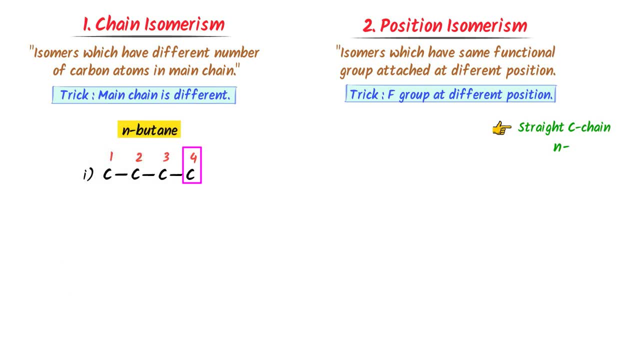 So this is n-butane. Now I will cut this carbon from the main chain and I will attach it at the second position. I get this structure Here: 1,, 2, 3.. This carbon is present at second position. Remember that. 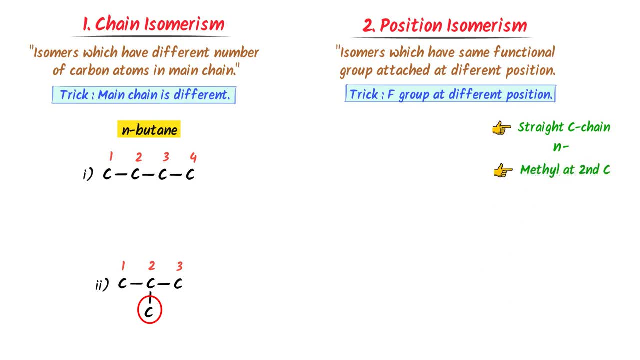 If methyl group is present at the second position, then this carbon is present at the second position. We call it iso. So this is isobutane. Now listen carefully. In this n-butane there are four carbon atoms present in the main chain, or parent chain. 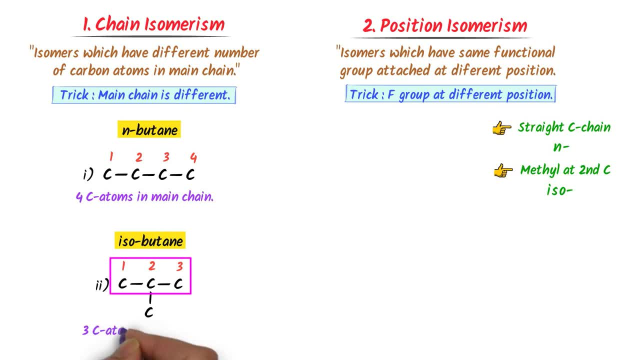 While in this isobutane there are three carbon atoms present in the main chain or parent chain. According to this trick, these isomers have different carbon atoms in the main chain, So they are chain isomers. Thus we write: 1 and 2 are chain isomers because they have different number of carbons present. 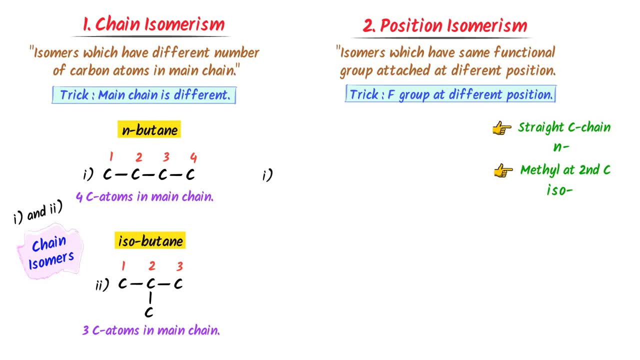 in the main chain or parent chain. Now consider pentane. I only consider the straight chain of pentane. We call this n-pentane. Secondly, I cut this carbon and I attach it to this second carbon, So this is n-pentane. 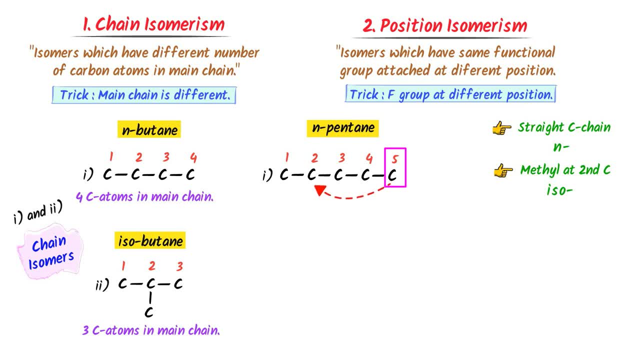 Now consider pentane. I only consider the straight chain of pentane. We call this n-pentane, So this is n-pentane. I only consider the straight chain of pentane and I attach it to this second carbon, I get this structure. 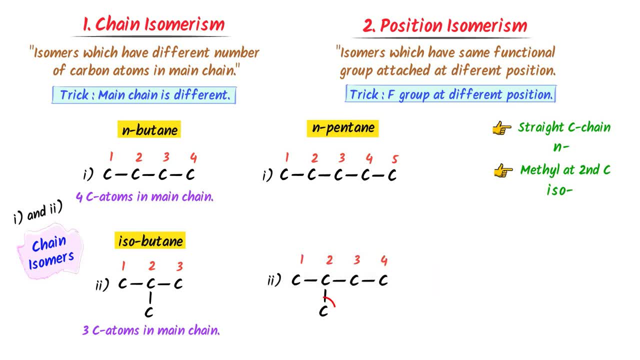 Here: 1, 2, 3, 4.. The methyl is present at the second carbon. I call it isopentane. Thirdly, I cut this carbon and I attach it to this second carbon. I get this structure Here: 1, 2, 3.. 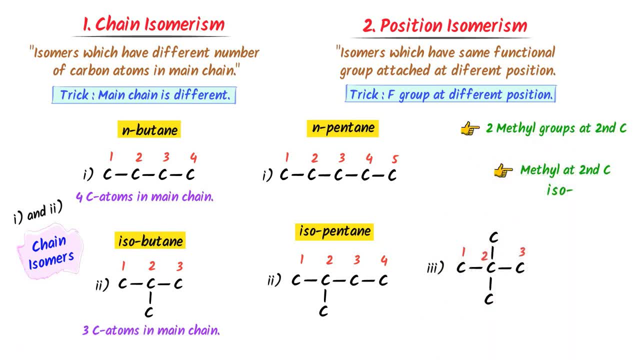 Remember that if there are two methyl groups present at the second carbon, we call this second carbon. Okay, it NEO, Hence this is neopentane. Now listen carefully. We can see that there are 5 carbon atoms present in the main chain of this compound. there are 4 carbon atoms present in the main. 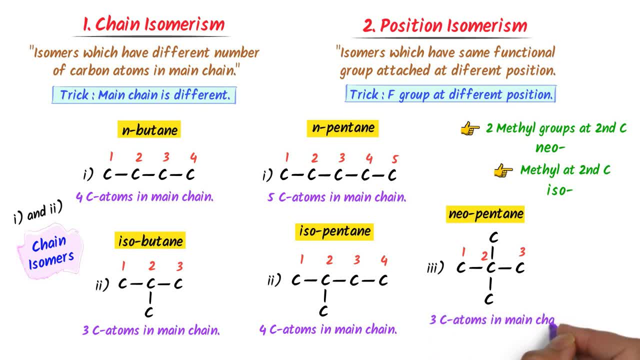 chain of this compound and there are 3 carbon atoms present in the main chain of this compound. According to this trick, these isomers have different carbon atoms and their respective chains, so they are chain isomers. Thus 1, 2 and 3 are chain isomers because they have 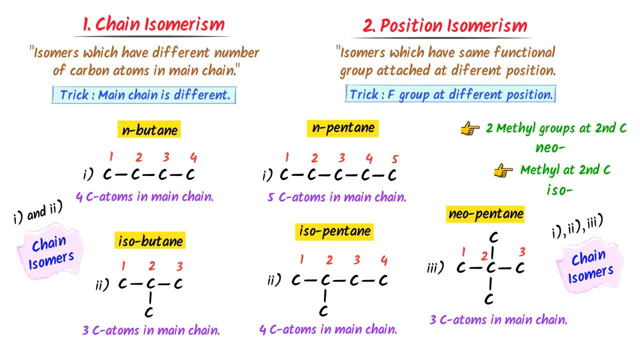 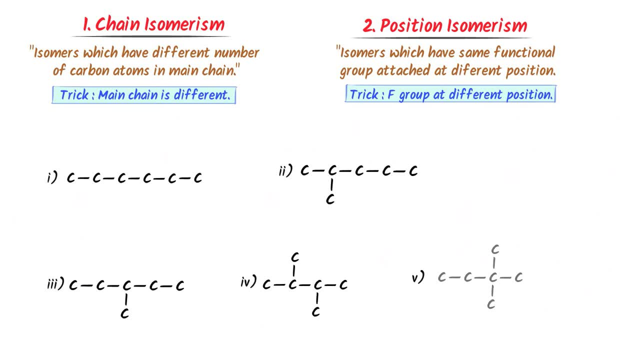 different number of carbons in the main chain or in the parent chain. Hence, note it down. Now consider these isomers of hexane. This is a straight chain of carbon atoms. There are 6 carbon atoms present in it. We call it N-Hexane. 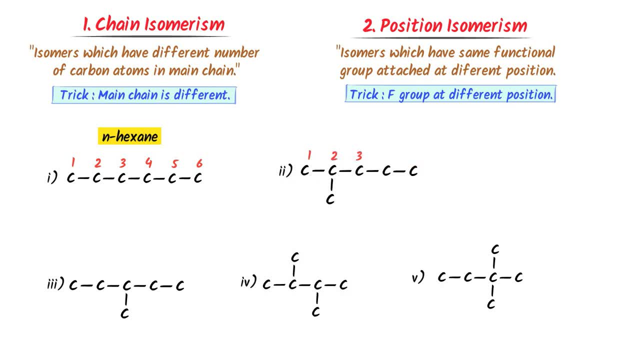 Secondly, I write 1,, 2,, 3,, 4, 5.. The methyl group is present at the second carbon. We call it Isohexane. Thirdly, I write 1,, 2,, 3,, 4, 5.. The methyl is present at the third carbon. I write 3-methylpentane. 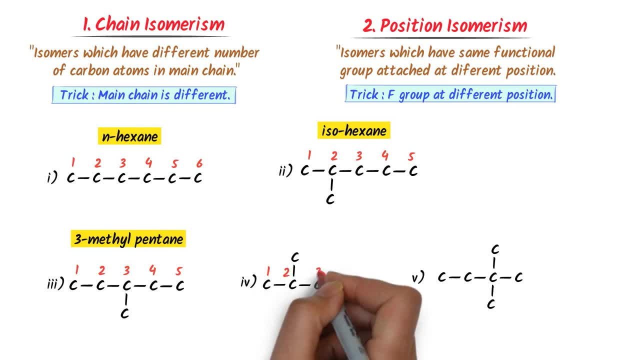 Fourthly, I write 1,, 2,, 3, 4.. One methyl is present at the second carbon And another methyl is present at the third carbon. I write 2, 3: dimethylbutane. Lastly, I write 1,, 2,, 3,, 4.. Here, two methyl groups are present at the second carbon. We 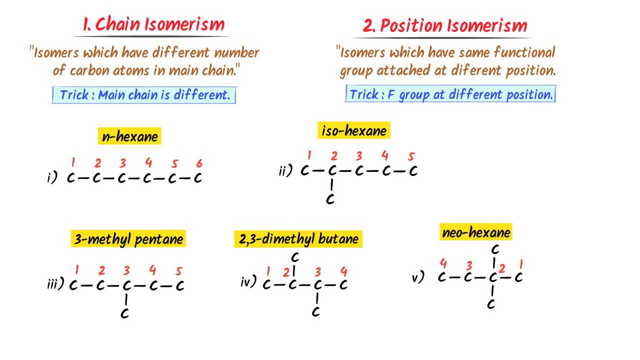 call it Nu-Hexane. Now I write the number of carbon atoms in the main chain 1: N2HH3.. There are 6 carbon atoms in the main chain 2, 2,, 3,, 4, 5.. There are 6 carbon atoms in the main chain There. 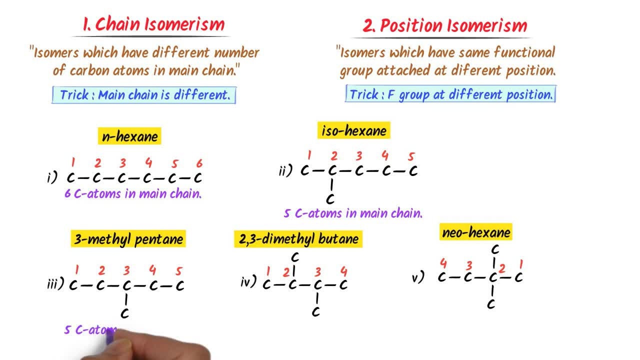 are 5 carbon atoms in the main chain: 2,, 2,, 3,, 4, 5.. Empty sodium is present in the main in the main chain. There are also 5 carbon atoms in the main chain. There are 4 carbon. 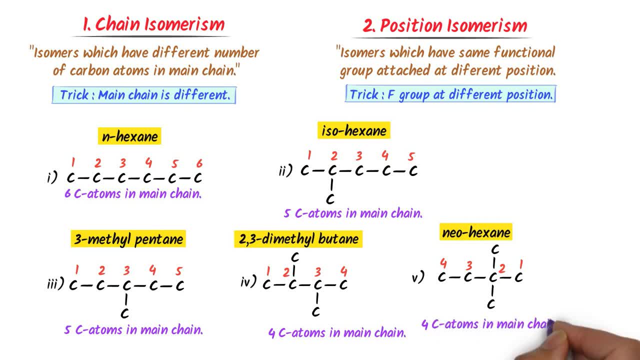 atoms in the main chain And there are also 4 atoms in the main chain. Now listen carefully. 1,, 2, and 4 are chain isomers, Because first isomer has 6 carbons in its main chain. 2 or 3. 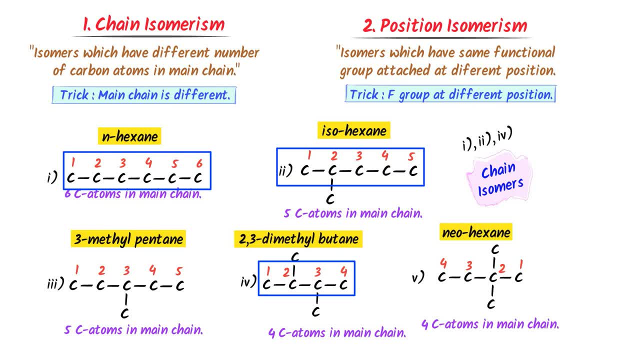 has 5 carbon atoms in its main chain, So we call it chain isomers. Secondly, we can see that 2nd and 3rd have 5 carbon atoms in the main carbon chain. They are not chain isomers. But wait a minute. Here the methyl group is present at the 2nd carbon While here 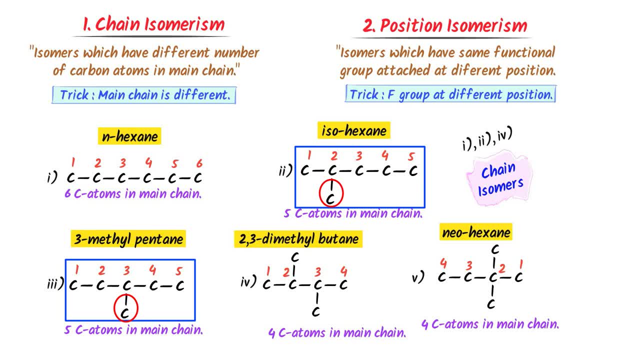 the methyl group is present at the 3rd carbon. According to the trick, the methyl group is present at the 2nd carbon And here the methyl group is present at the 3rd carbon. The main chain has 5 carbon atoms, But the functional group, CH3, is a different. 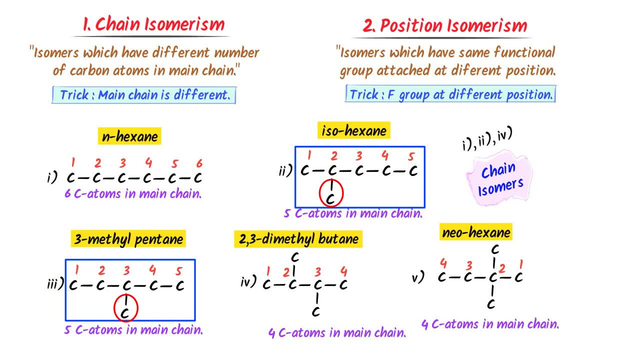 position, So they are position isomers. The 2nd and 3rd are position isomers. Similarly, in the 4th isomer the main chain, or parent chain, has 4 carbon atoms, While the 5th isomer 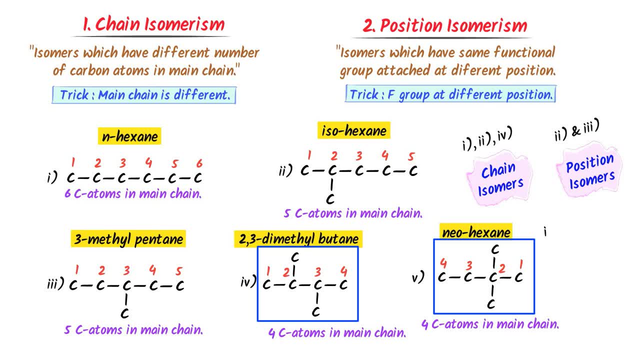 has also 5 carbon atoms in the main chain. Here the two methyl groups are present at the 2nd carbon and at the 3rd carbon, While here the two methyl groups are present at 2nd carbon. These both isomers have same carbon chains, But functional groups are present at 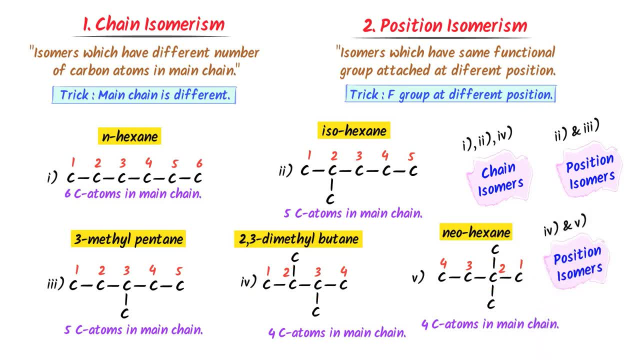 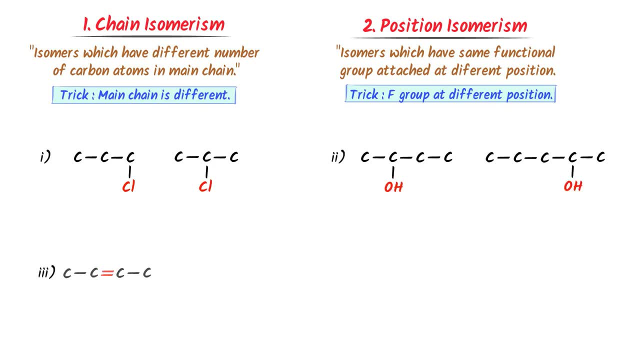 different position. Hence 4th and 5th are also position isomers. Hence note it down. Finally, consider these isomers. Pause the video and try to find the isomer. Well, they both have the same carbon chain, having 3 carbon atoms in the main chain, But here, 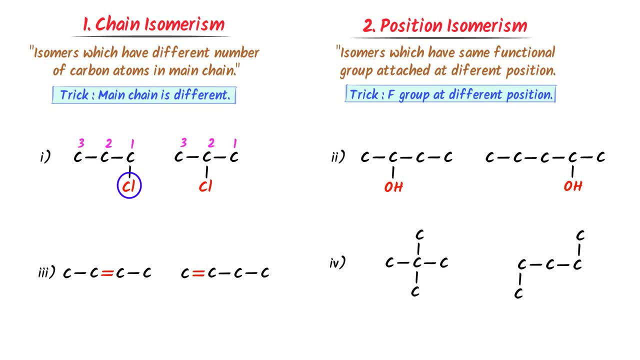 the chlorine is present at the 1st carbon And here the chlorine is present at the 2nd carbon. So they are position isomers. Secondly, this compound has 4 carbon atoms in the main chain And this compound has 5 carbon atoms in the main chain. So they are position isomers. 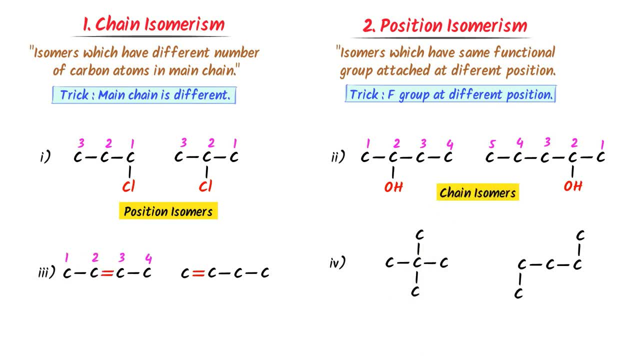 And these are chain isomers. Thirdly, the double bond is present at the 2nd carbon, While here the double bond is present at the 1st carbon. So they are position isomers. Fifthly, the main chain has 1-2-3 carbon atoms, While here 1-2-3-4-5.. 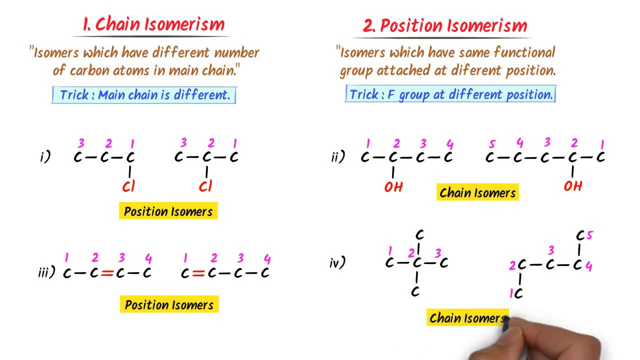 Here are 5 carbon atoms, So they are chain isomers. Therefore, Remember that chain isomers have different number of carbon atoms in the main chain, while position isomers have the same functional group bonded at different position in the same carbon chain. 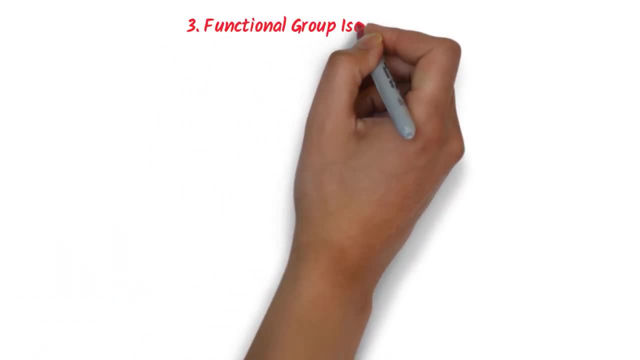 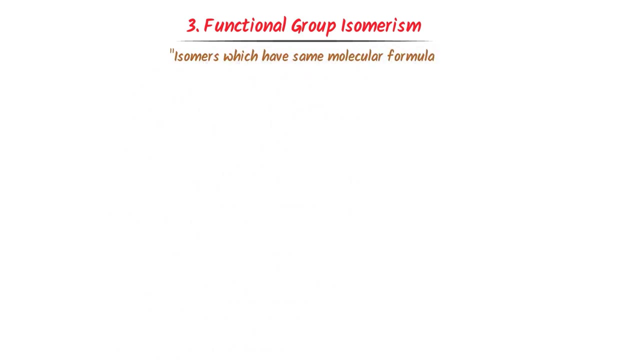 Now we will learn the third type of isomerism, which is known as functional group isomerism. Well, those isomers which have same molecular formula but different functional groups are called functional group isomerism. In order to spot functional group isomerism, always look at these. 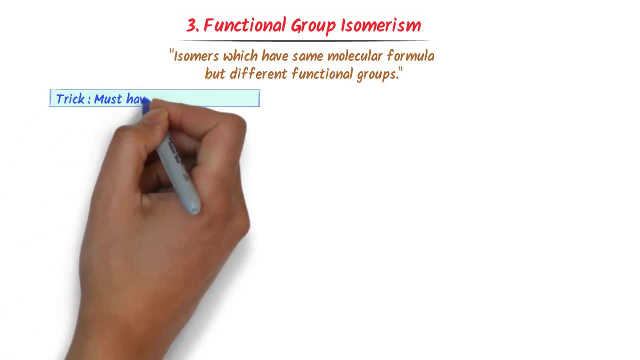 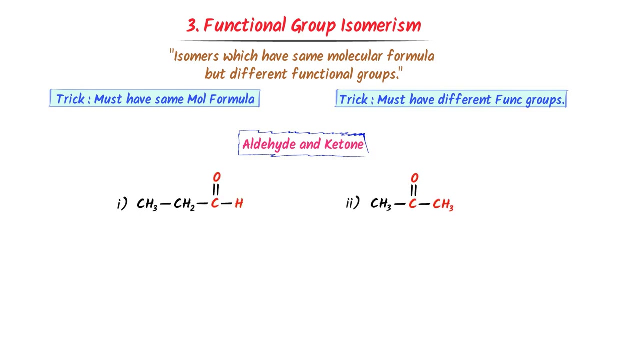 two conditions. Firstly, the two compounds must have the same molecular formula. Secondly, the two compounds must have different functional groups. For example, consider aldehyde and ketone functional group. Now I look for the molecular formula of the compounds, The molecular formula. 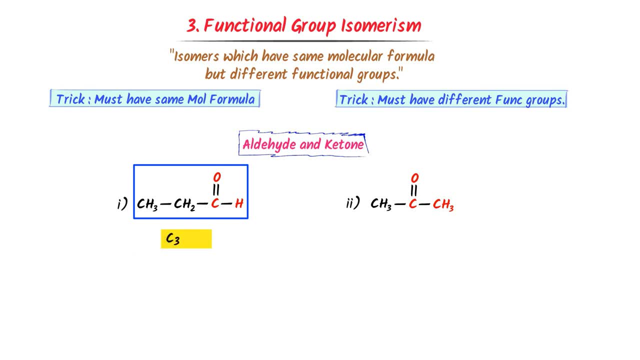 of this aldehyde is: there are three carbon atoms, six hydrogen atoms and one oxygen atom. The molecular formula of this ketone is: there are also three carbon atoms, six hydrogen atoms and one oxygen atom. Secondly, the functional group of aldehyde is COH. 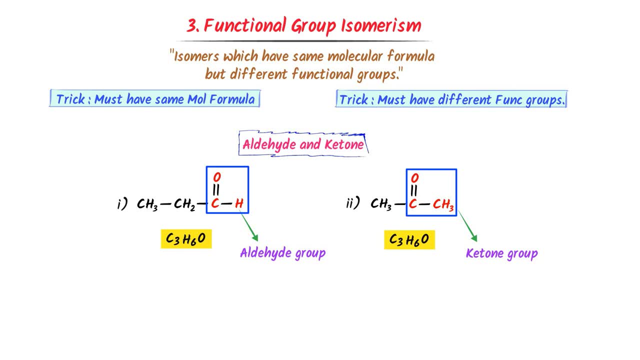 and that of ketone is COCH3. They both have different functional groups. Thus this aldehyde and this ketone are functional group isomers of each other. Now consider carboxylic acid group and easter functional group. as usual, I look for the molecular. 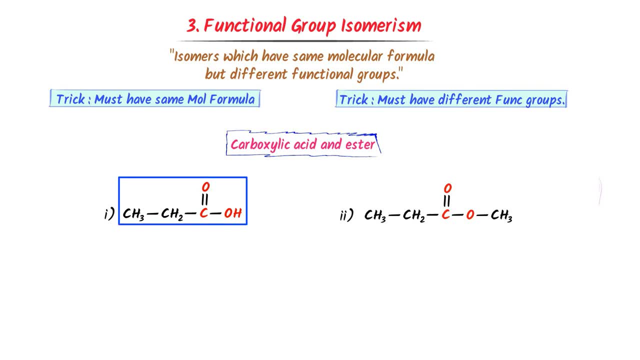 formula of the compounds. In this carboxylic acid there are three carbon atoms, six hydrogen atoms and two oxygen atoms, while in this easter are also three carbon atoms, six hydrogen atoms and two oxygen atoms. Secondly, the functional group of carboxylic acid is COOH and that of ester is COO. They both have different functional groups. 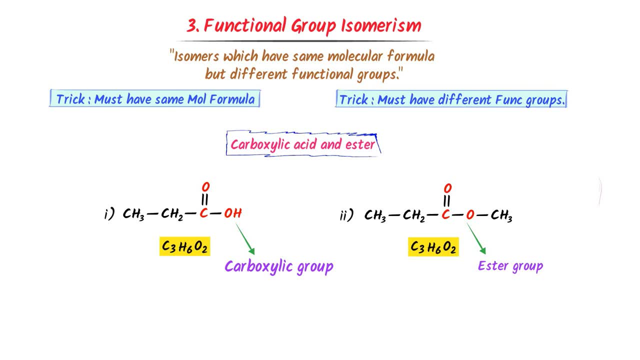 so both the conditions are fulfilled. Thus this carboxylic acid and this ester are functional group isomers of each other. Now consider ether functional group and alcohol functional group. As usual, I find the molecular formula of compounds. In this ether compound there are two. 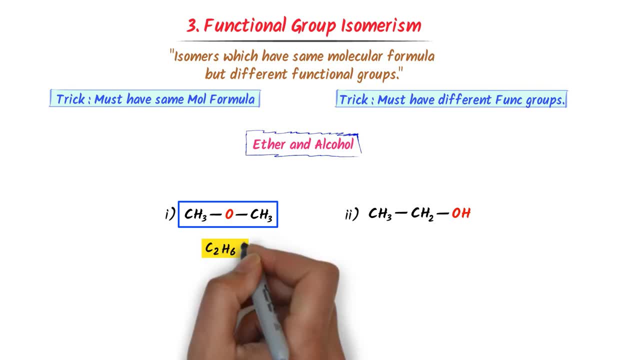 carbon atoms, six hydrogen atoms and one oxygen atom, While in this alcohol compound there are also two carbon atoms, six hydrogen atoms and one oxygen atom. Secondly, the functional group of ether is O And that of alcohol is OH. They both have. 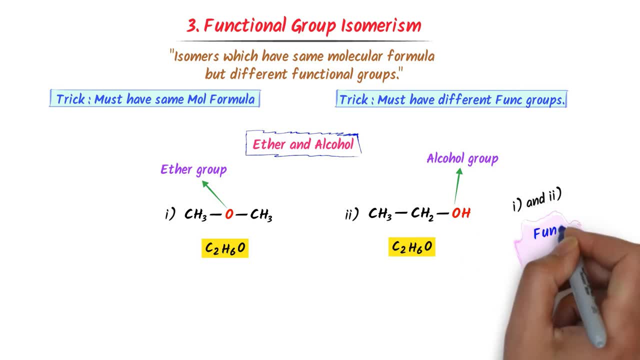 different functional groups. Thus this ether and this alcohol are functional group isomers of each other. Lastly, consider alkene functional group and cycloalkane functional group. I find the molecular formula of these compounds In the alkene there are: 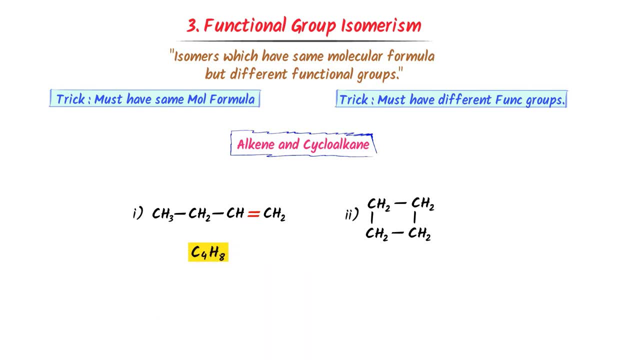 are four carbon atoms and eight hydrogen atoms, While in this cycloalkane there are also four carbon atoms and eight hydrogen atoms. Secondly, the functional group of alkene is double bond and that of cycloalkane is single bond. Both the conditions are fulfilled. Thus this alkene 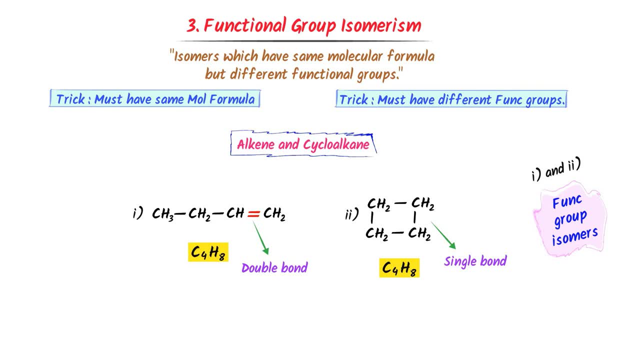 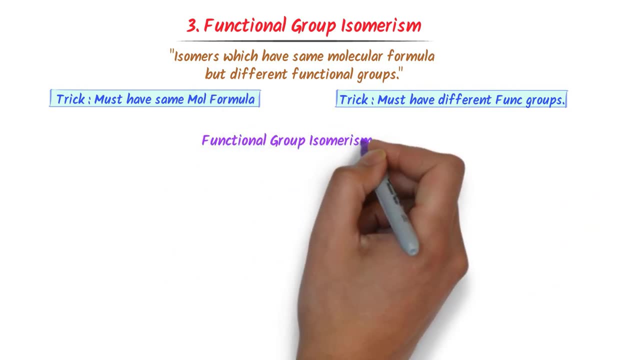 and this cycloalkane are functional group isomers of each other. To summarize this whole concept, we have learned that functional group isomerism exists between aldehyde and ketone, carboxylic acid and ester ether and alcohol, alkene and cycloalkane. Thus, remember that 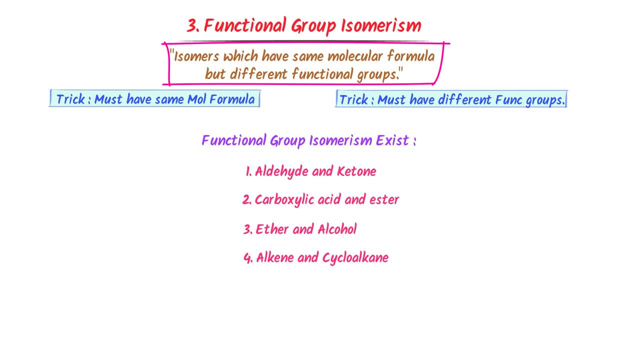 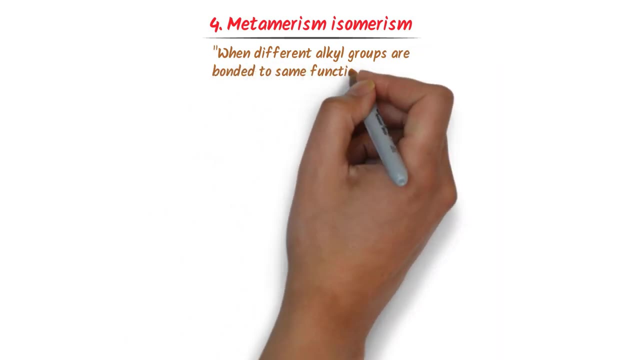 functional group isomers are those isomers which have same molecular form as the cycloalkane. Thus, remember that functional group isomers are those isomers but different functional groups. Now we will learn the four type of isomerism, which is metamerism? Well, when different alkyl groups are bonded to the same functional group, 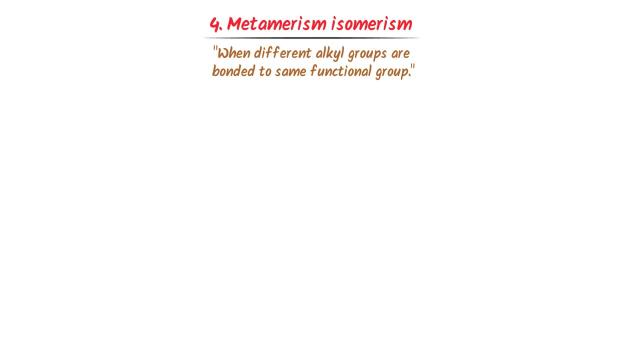 are called metamerism. The condition is same: functional groups and different alkyl groups. Here the question is: what are alkyl groups? Well, consider methane CH4. When we remove one hydrogen from methane, we get CH3 and we call it methyl. Secondly, 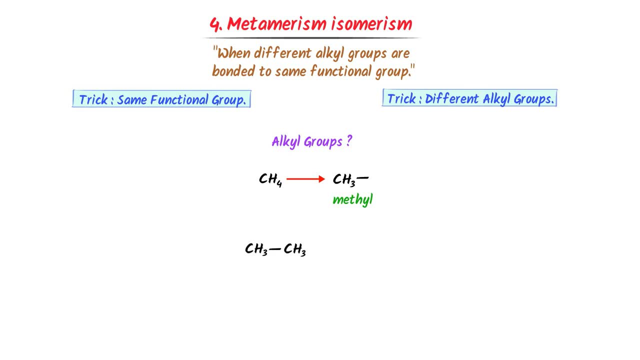 consider ethane: When we remove one hydrogen from it, we get CH3CH2 and we call it ethyl. Thus, by this way, we can form alkyl groups. Remember that alkyl group is represented by R' Now consider ether functional group. The ether group is R' O' R Here. let, this is the left-hand. 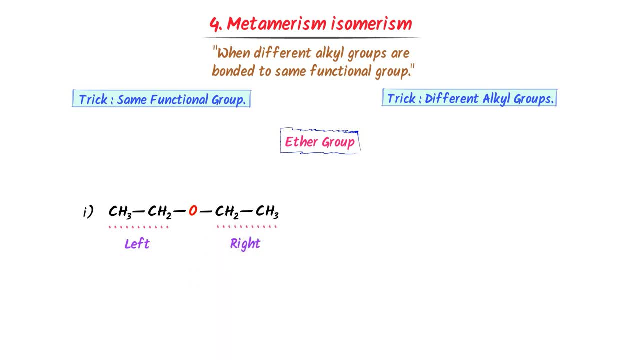 side of this ether, and this is the right-hand side of this ether. At the left side there is ethyl, while at the right side there is also ethyl. This ether contains two ethyl groups. We call it diethyl ether. 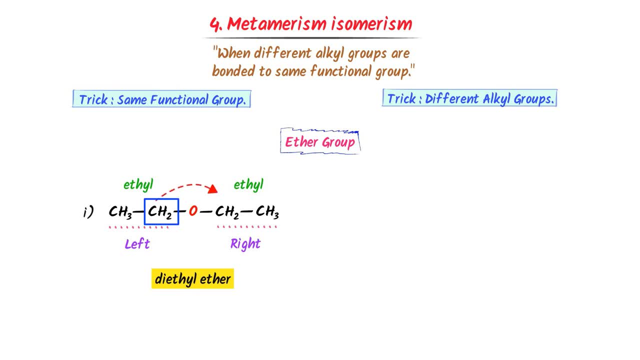 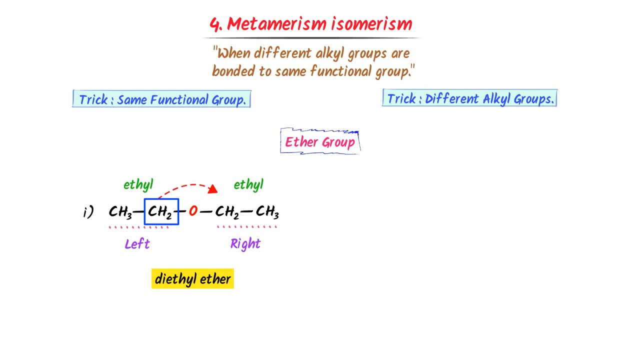 repeat it: I shift this CH2 from the left side to the right side, I get this new compound Here. in this compound, this is the left side and this is the right side. At the left side there is methyl group, While at the right side there is propyle. 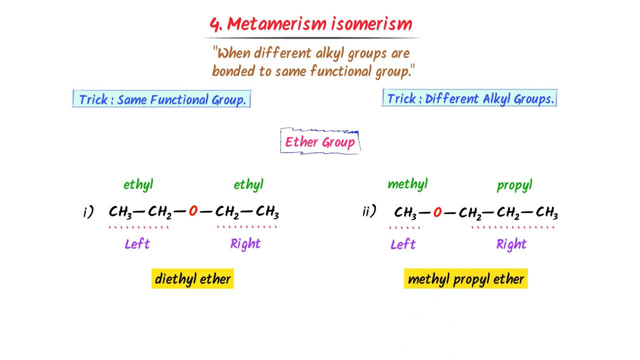 group. I write methyl propyle ether. Now listen carefully. These two compounds have the same functional group, which is ether, but at the left side of this molecule there is ethyl, while at the left side of this molecule there is methyl. 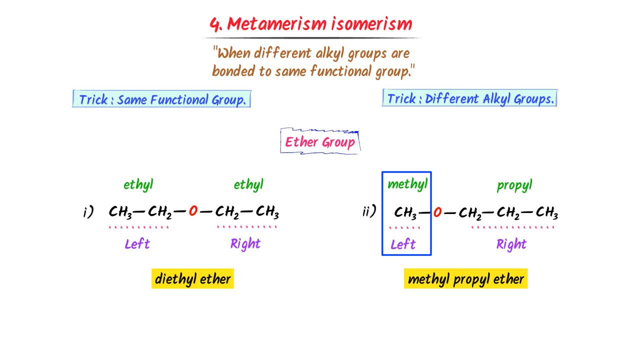 According to the condition, these molecules have same functional group, but different alkyl groups are attached to it. Thus we call them two metamers of each other or two isomers of each other, hence noted down. Now consider amine functional group: 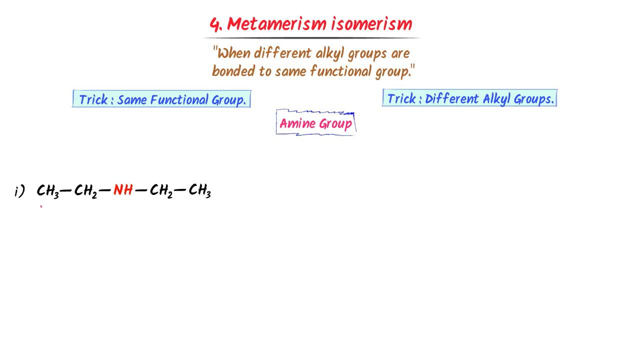 We know that the functional group of amine is R-NH-R- Let. this is the left side of this compound and this is the right side of this compound. At the left side there is ethyl group and at the right side there is also ethyl group. 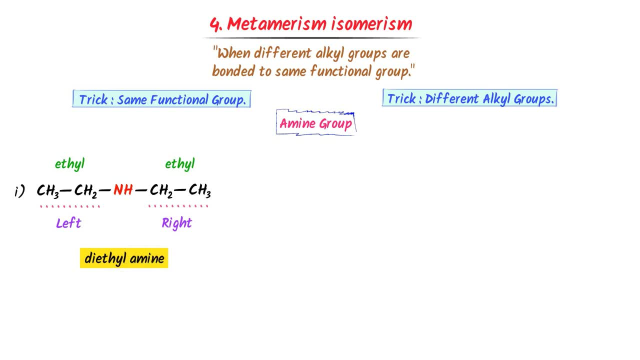 So we call it diethylamine. Now I shift this CH2 from the left side to the right side. I get this new compound Here. at the left side There is methyl group, while at the right side there is propyl group. 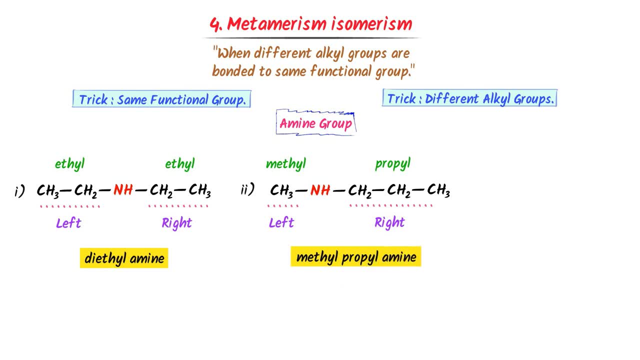 So we call it methyl propylamine. Lastly, I cut these two carbons of the propyl. I attach it to this carbon. I get this new compound Now. at the left side there is methyl group, while at the right side there are two methyl. 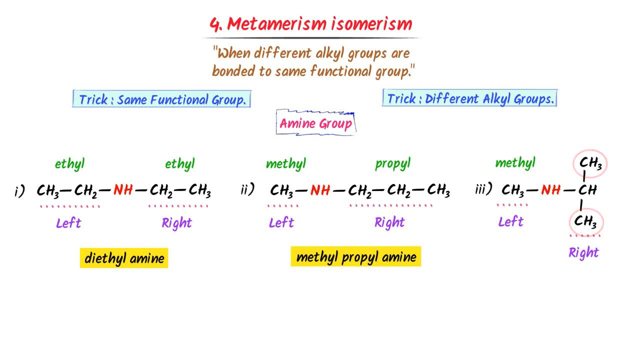 groups bonded to second carbon. We call it isopropyl. Thus we get methyl isopropyl amine. Now listen carefully. These three compounds have the same functional groups, which is amine, NH. At the right side of this compound there is ethyl. 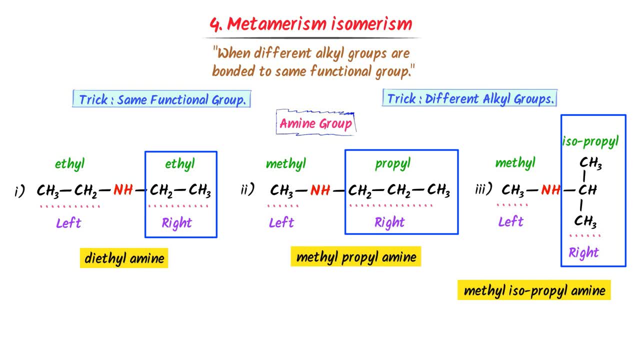 And at the right side of this compound there is isopropyl. Hence the condition is fulfilled. Thus, these three are metamers, Are three isopropyls. They are the isomers of each other, So note it down. 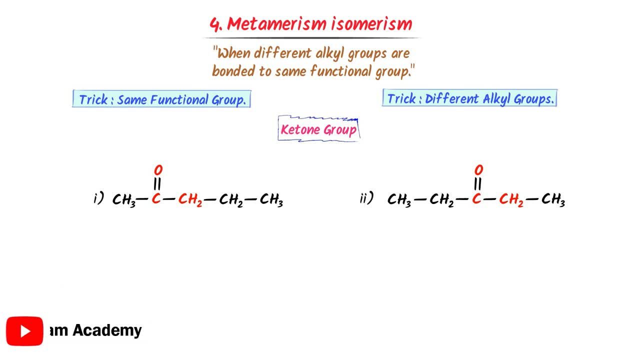 Finally, consider ketone functional group. We know that its functional group is R'CO'R. Now consider these two compounds. Pause the video and try to find its isomerism. Here I write 1,2,3,4,5.. 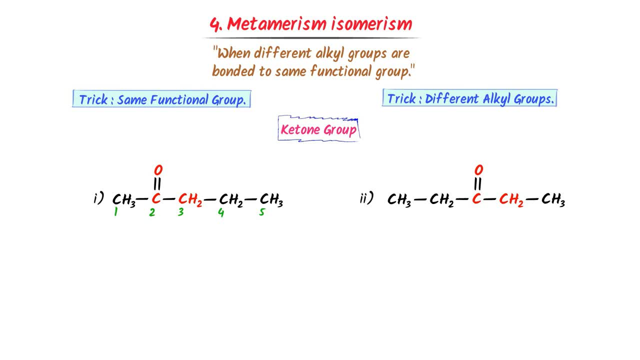 The functional group of ketone is present at the second carbon, So we call it isomerism. Now listen carefully. At the left side of this compound there is ethyl group, While at the left side of this compound there is methyl group. 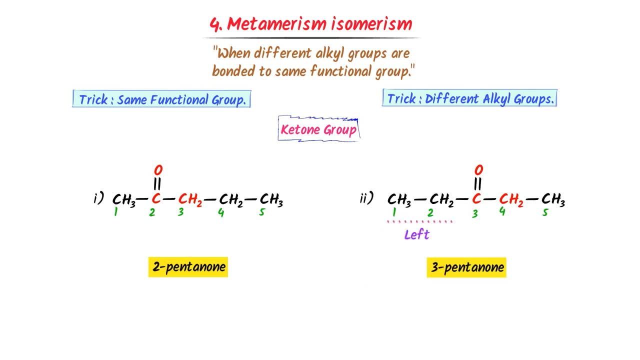 Hence they both are metamers or isomers of each other. Thus, remember that if compounds have same functional group but different alkyl groups are bonded to it, it is known as metamorism. To summarize this: we have two compound, We have one isopropyl. 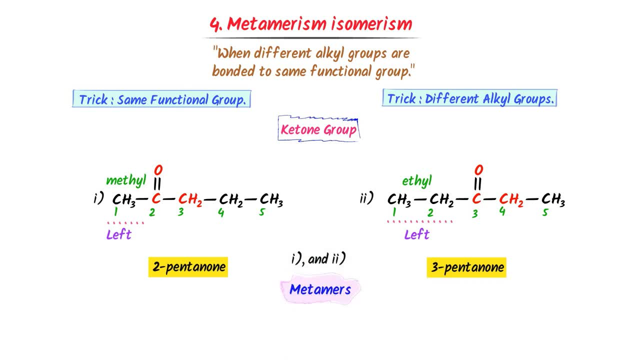 Two isopropyls- One isopropyls And two isopropyls. We have two isopropyls. So we have two isopropyls And we have two isopropyls. 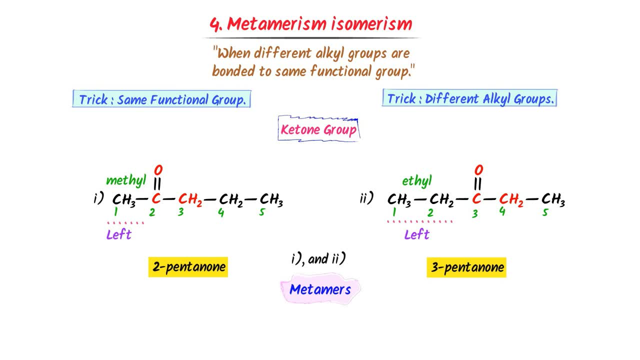 We have two isopropyls And we have two isopropyls And we have two isopropyls And this is a group of isopropyls, whole concept. we have learned that metamerism is possible in ether functional group amine. 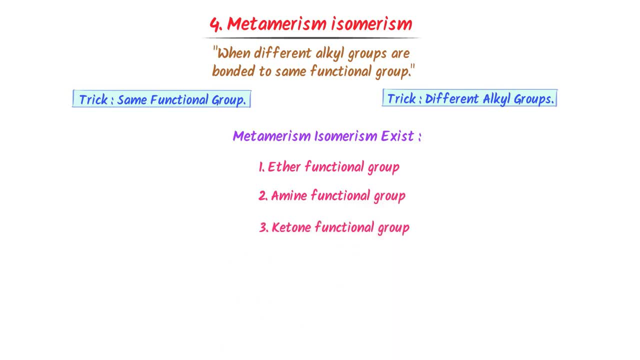 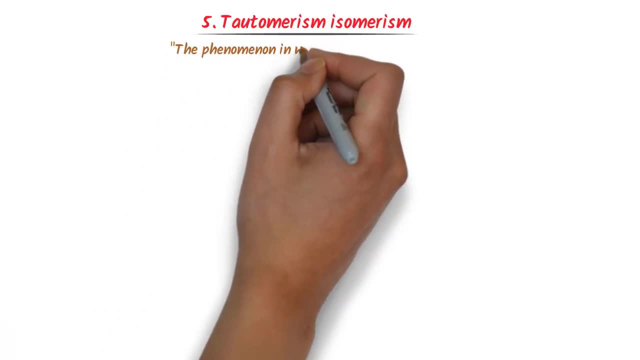 functional group and ketone functional group. Now we will learn the fifth type of isomerism, which is tautomerism. The phenomena in which single compound exist and two are more interconvertible structures are called tautomerism. Remember that tautomerism is possible in carbonyl. 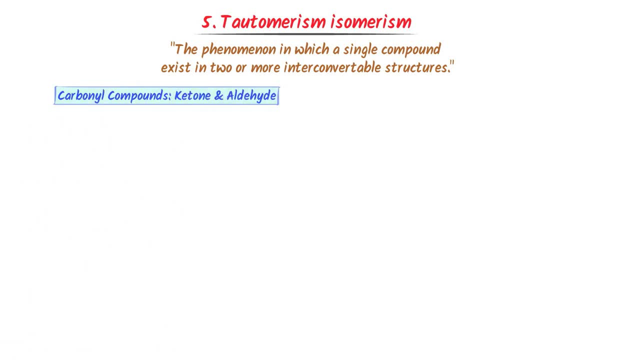 compounds having CO group, like ketone and aldehyde. Personally, I teach this condition for tautomerism. It is CH. If any compound has this pattern, there is 90% chances that tautomerism will occur. Here I write 1,2,3.. I shift hydrogen from first position to the third. 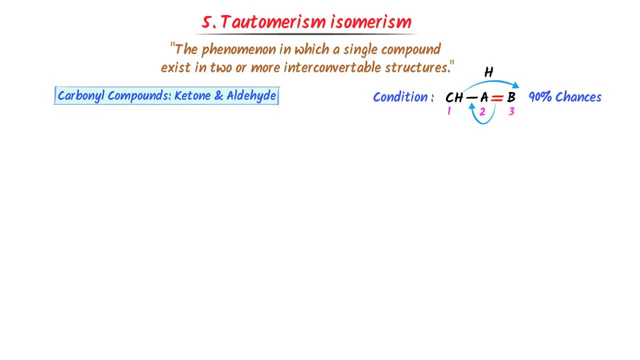 position and I shift double bond from second position to the first position. Thus, using this conversion, we can easily do tautomerism of any compound. For example, consider this ketone. Here this carbon double bond due to oxygen is like A. double bonded to B, I write AB. This CH3 is like CH, So the condition: CH. 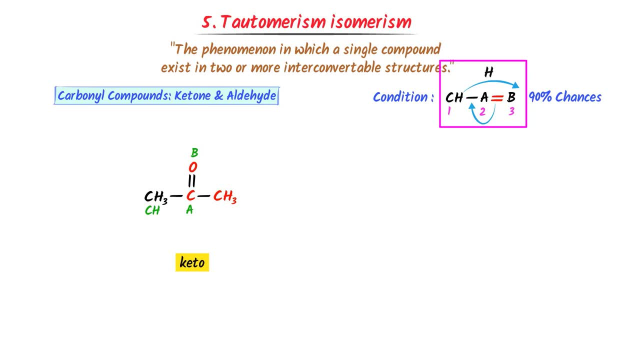 single bond, A, double bonded to B, is fulfilled. Hence tautomerism is possible in this organic compound. I write 1,2,3.. Now, according to the condition, I shift: hydrogen from first position to the third position, I shift. hydrogen from first position to the third position, I shift. 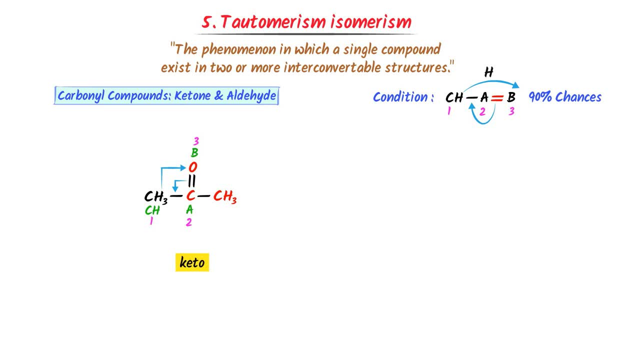 hydrogen from first position to the third position And I shift double bond from the second position to the first position. I write CH2, because I shift one hydrogen Double bond, carbon single bond, OH and CH3.. This compound contains double bond of alkene. I write En, And for this OH I write Ol. 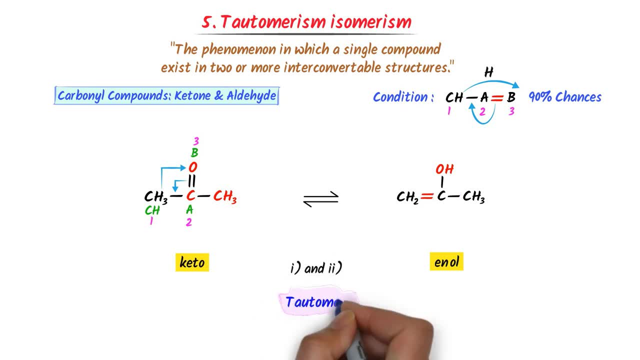 So I get Enol. Hence these are the two tautomers, or two isomers of each other. Remember, we also call tautomerism as keto-enol isomerism, because we get ketone and enol. This double arrow means that ketone and enol are in dynamic equilibrium. 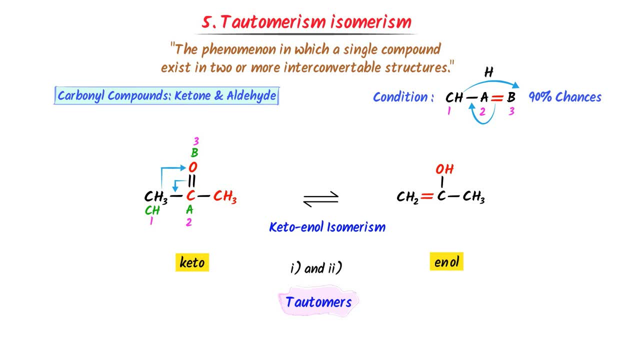 They are interconvertible. That's why we also call it dynamic isomerism, because they are moving from one form or from one structure to another structure. Remember that we will get 99% of ketone and 1% of enol, because ketones are very stable than enol. 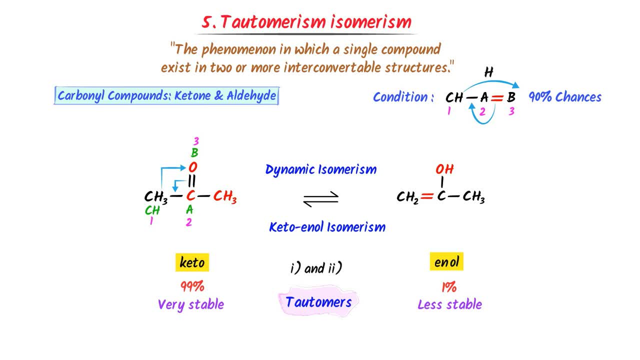 Let me repeat it: Ketones are very stable than enol. Now consider this aldehyde Here. this carbon double bonded to oxygen is like A double bonded to B. I write A and B. This CH3 is like CH. The condition CH single bond, A double bonded to B is fulfilled. 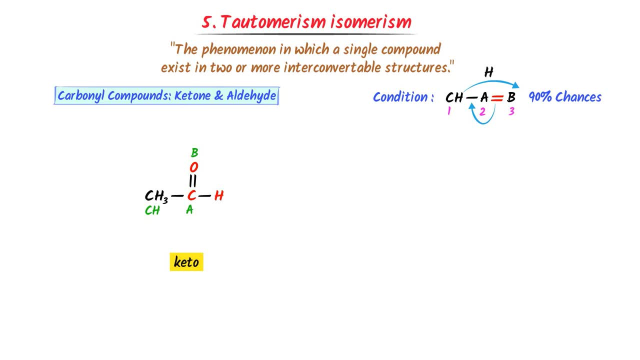 Hence tautomerism is possible in this compound. I write 1,, 2,, 3.. Now, according to the condition, I shift hydrogen from the first position to the third position and double bond from the second position to the first position. As a result, I get CH2 double bond, C single bond, OH. 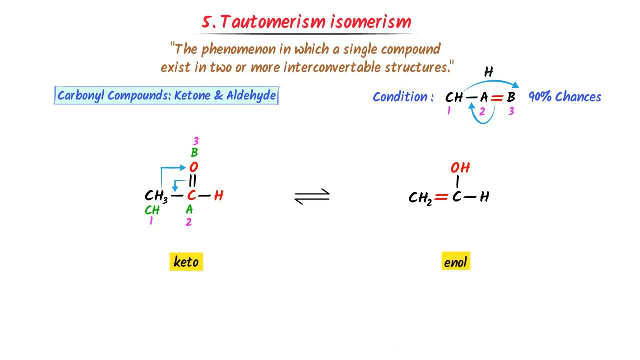 and H. This is enol. As usual, we get 99% of aldehyde and 1% of enol. Hence, these are the two tautomers, or two isomers of each other. Now consider this organic compound. Pause the video. 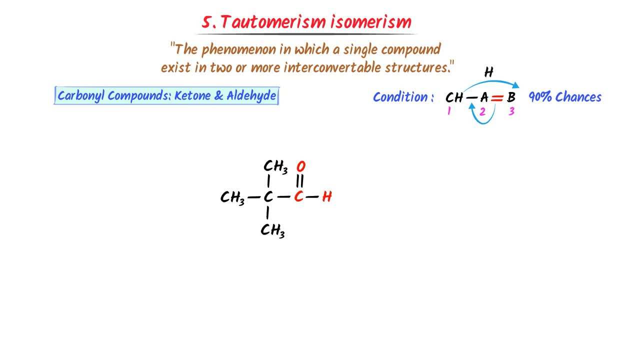 and try to find its tautomers. Well, this C double bonded to oxygen is like A double bonded to oxygen. I write A and B. This carbon has no hydrogen. Here the CH is not present. I mean this carbon has no hydrogen. The condition CH single bond, A double bonded to B is not fulfilled. 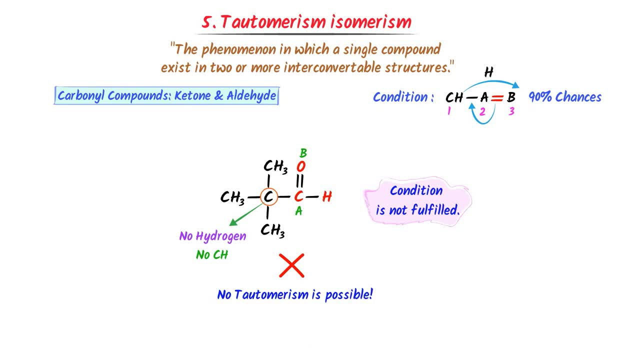 The tautomerism is not possible in this compound. Now consider this organic compound. This N double bonded to O is like A double bonded to B. I write A and B. This CH2 is like CH. The condition CH single bond, A double bonded to B is fulfilled. I write 1, 2, 3.. I shift hydrogen from the first. 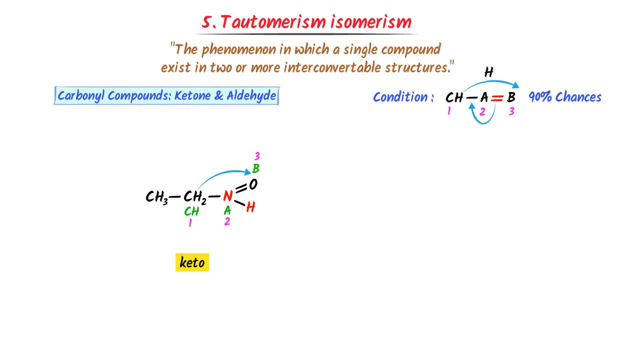 position to the second position And I shift double bond from the second position to the first position. As a result, I get this compound. Thus, by this way, we can easily do tautomerism of organic compounds. Now we will learn the exception cases of tautomerism. Usually these exception- 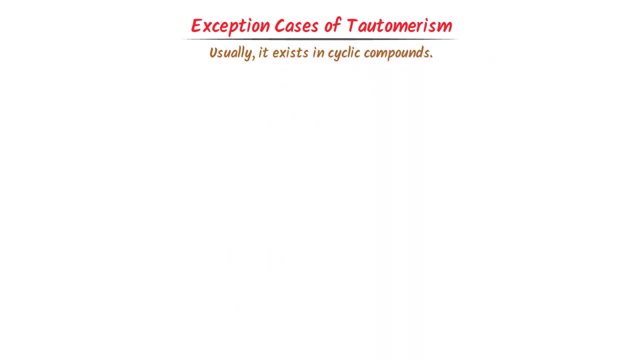 cases exist in cyclic organic compounds. For these cases we can use the Tautomerism method. We have to learn two important concepts: Aromatic, anti-aromatic and conjugation. For aromatic and anti-aromatic compounds I use this trick: I write 2 and 4.. Now I increase both. 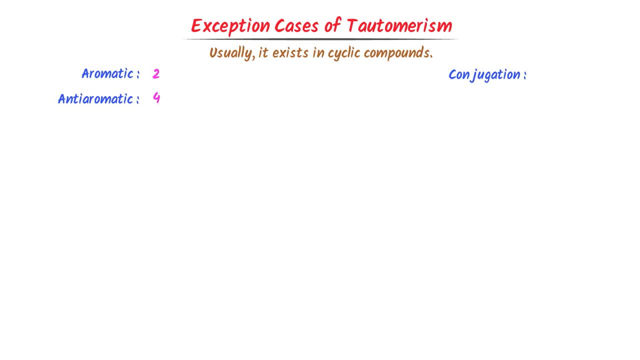 the numbers by 4.. 2 plus 4 is equal to 6.. 6 plus 4 is equal to 10, and so on. Here, 4 plus 4 is equal to 8.. 8 plus 4 is equal to 12, and so on. Remember that these numbers represent the total number of. 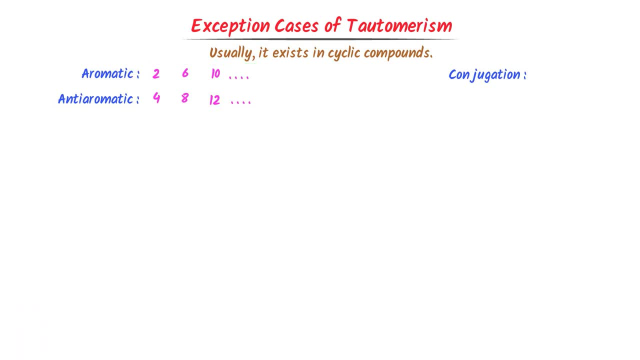 electrons. Also noted down that if there is negative charge, it represents two electrons, If there is a lone pair, it represents two electrons And if there is double bond, it also represents two electrons. On the other hand, if there is a 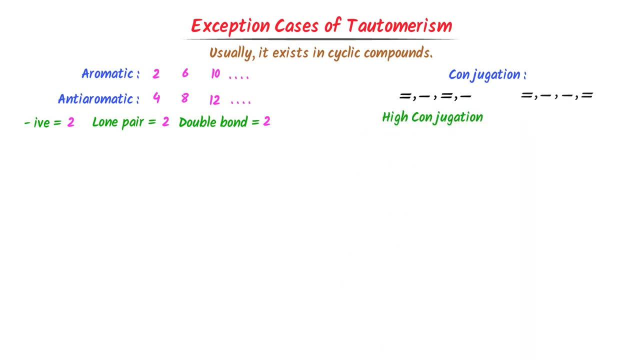 alternate single and double bond, it shows high conjugation. So on the basis of these two concepts we will easily learn the exception cases of tautomerism. The first exception case is chsinglebond to b. Here this condition exists but tautomerism is not exhibited by the compound, For example: 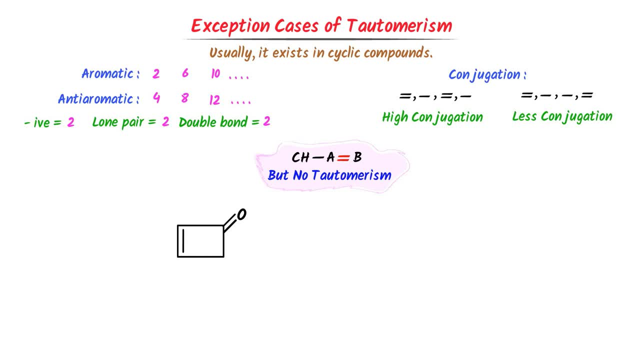 consider this organic compound. Firstly, I write CH, C and CH2.. This C double bonded to O is like A double bonded to B, And this CH or this CH2 is like CH. So the condition CH single bond, A double bonded to B is fulfilled. 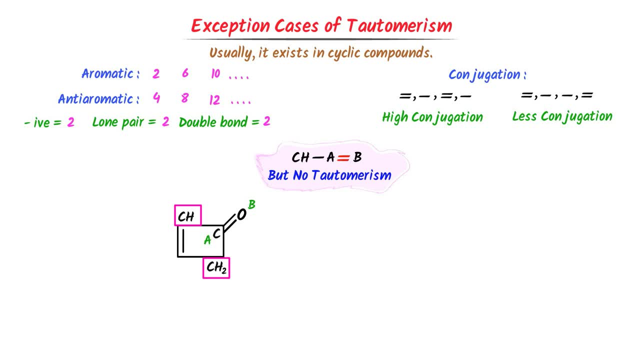 I can take both this CH or this CH2, but I consider this CH2.. Here this H of CH2 is shifted to third position and the double bond is shifted to the second position. I get this compound, But wait a minute. we know that these both compounds are cyclic. 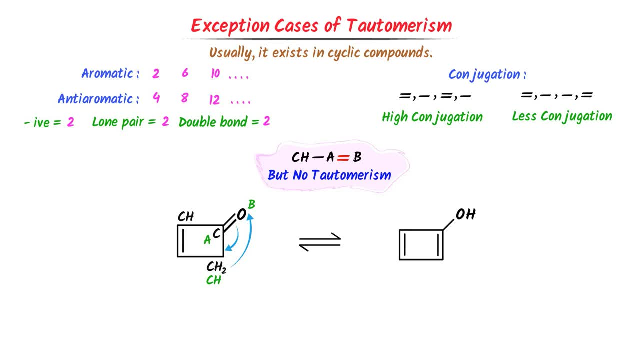 So I have to check either these compounds are aromatic or anti-aromatic. So I have to check either these compounds are aromatic or anti-aromatic. So I have to check either these compounds are cyclic or anti-aromatic. This cyclic compound has one double bond. 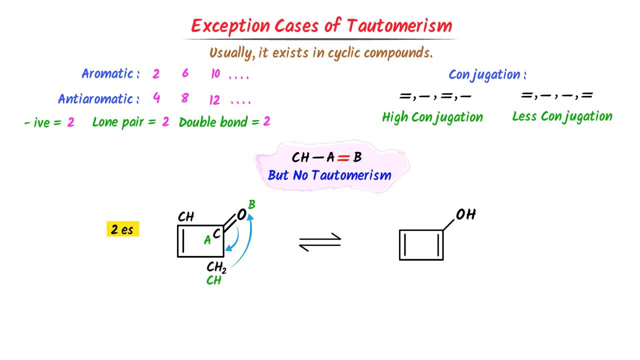 I write two electrons. We know that if a compound has two electrons, it is aromatic. Hence this compound is aromatic. On the other hand, this compound has two double bonds. I write 2 plus 2.. I get four electrons. We know that if a compound has four electrons, it is anti-aromatic. 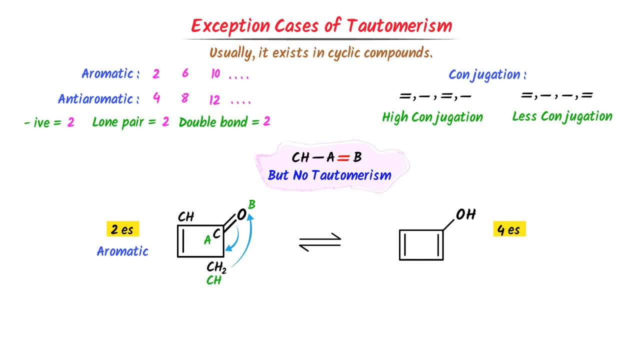 Hence, this compound is aromatic. Now listen carefully. Aromatic compounds are very stable, whereas anti-aromatic compounds are less stable. So this compound does not exist because it is anti-aromatic and it is less stable. As a result, we get 100% of this compound. 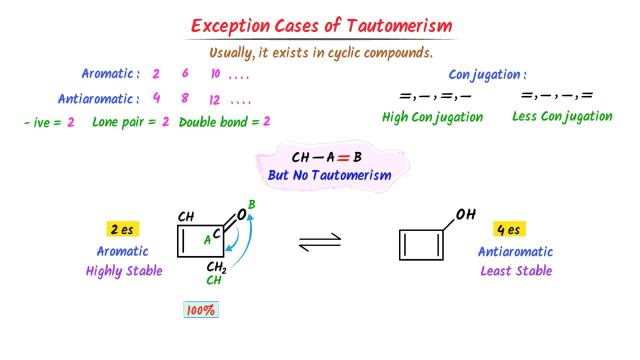 This compound is aromatic and it is very stable compound. On the other hand, we get 0% of this compound because it is anti-aromatic and it is less stable. As usual, this is ketone part and this is enol part. We get greater ketone part and lesser enol part. Therefore, we say that this compound 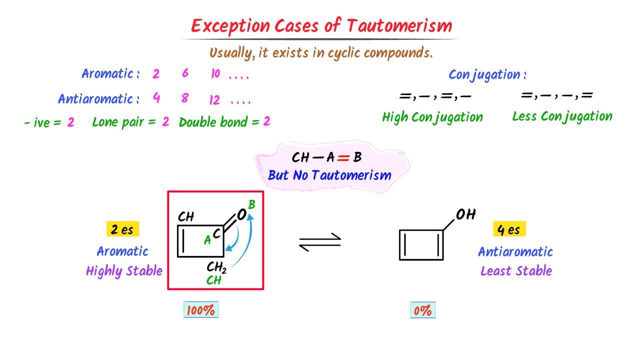 does not exhibit tautomerism, even though it fulfilled the condition CH. single bond, A double bonded to B. Hence noted down this exception case. Secondly, enol part is greater than ketone part. We have learned that we always get greater ketone part and lesser enol part, But in this exception case we will get greater enol part. 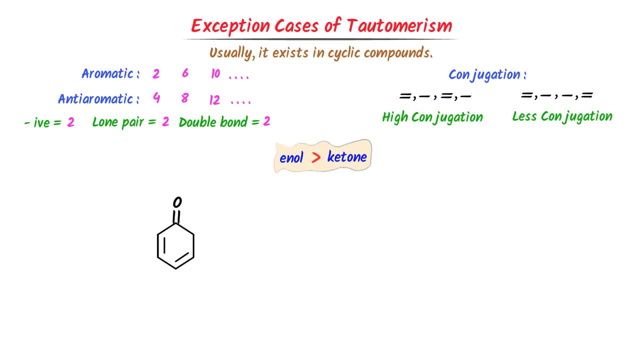 and lesser ketone part. Let's consider this example. I write C and CH2.. This C double bond, O is like A, double bonded to B, while this CH2 is like CH. The condition is satisfied. I shift hydrogen to this third position and the double bond to the first position. As a result, I get this: 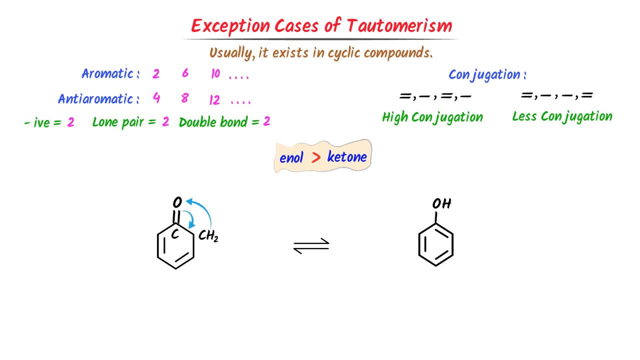 compound. These both compounds are cyclic. I check aromatic and anti-aromatic compounds. This compound has two double bonds. I write: 2 plus 2 is equal to 4 electrons. We know that if there are four electrons it is an anti-aromatic compound. Thus this compound is anti-aromatic and it is less. 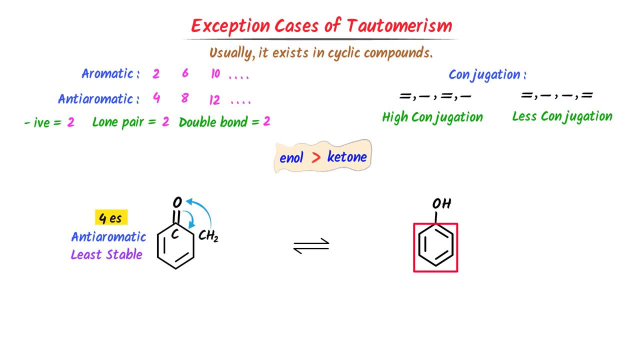 stable, While this compound has three double bonds. I write Baending power 1 and B Wr billionaire, for a total of B and 1 ToR. What we get here is this compound shows that the antiromatic compounds have better acidity level over earth. Then I subtract: 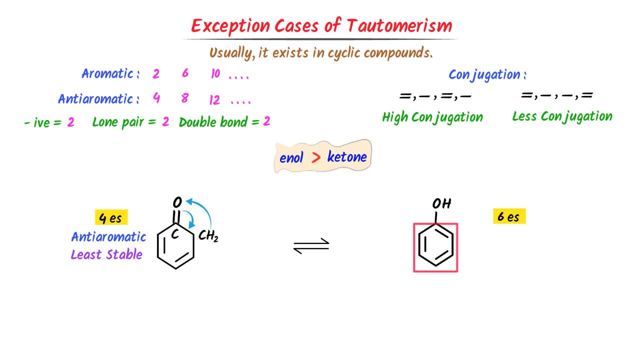 2 plus 2 is equal to 6 electrons. We know that if there are 6 electrons, it is aromatic compound. Thus, this compound is aromatic compound and it is highly stable. So we get 100% of aromatic compound because it is highly stable, while we get 0% of anti-aromatic compound because it is. 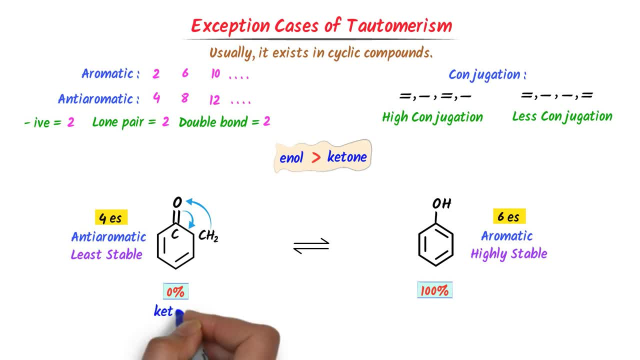 less stable. We know that this is ketone part and this is enol part. Hence we get greater percentage of enol part than ketone percentage. Thus, note it down, this exception case. Thirdly, consider this exception case when there are two possible isomers. Firstly, I write CH3C, CH2C and CH3. 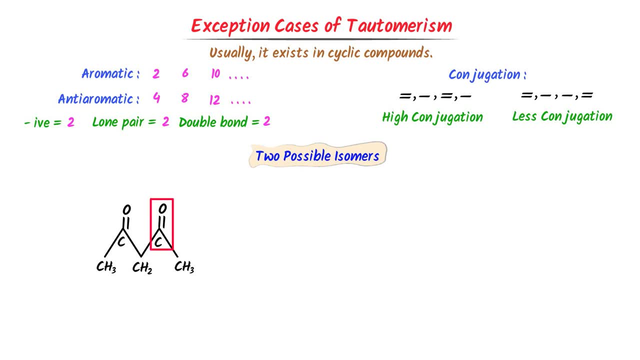 Now this C double bonded O is like A double bonded to B. This CH2 and this CH3 are like CH. Let this CH3 gives its hydrogen to this oxygen. The double bond will shift. here I get this compound. Secondly, let this CH2 gives its hydrogen to this oxygen. This double bond shifts. 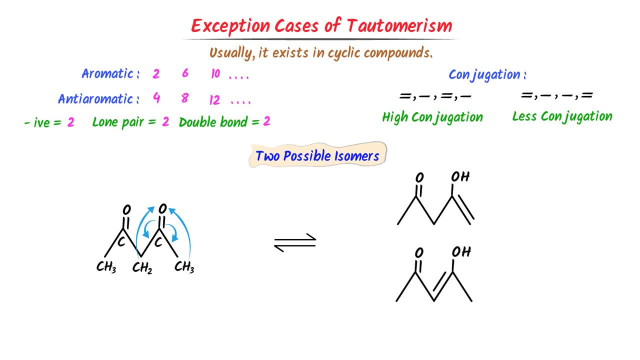 here I get this compound. Now listen carefully. this compound has single bond, double bond, single bond, single bond, double bond, while this compound has single bond, double bond, single bond, double bond, etc. We know that if a compound has alternate single and double bond, it is more conjugated and 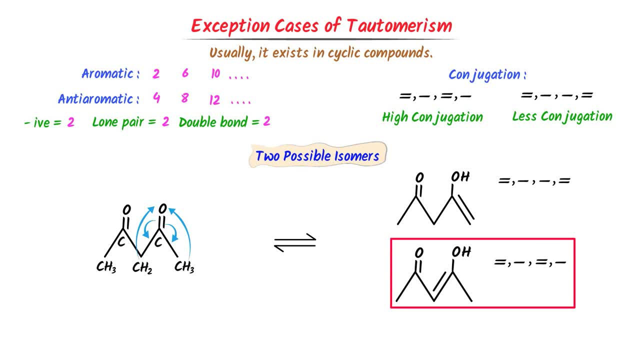 more stable. This compound has alternate single and double bond. it is more conjugated and more stable, While this compound has not alternate single and double bond, it is less conjugated and less stable. Thus, we will get greater content of this compound. 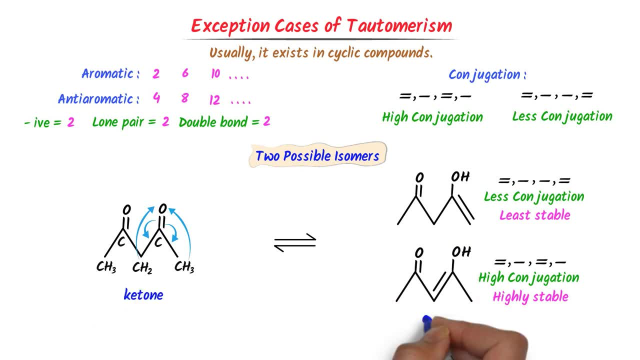 We know that this is ketone part and this is enol part. I get 85% of ketone part and 15% of enol part. Hence noted down this exception case. Therefore, using aromatic, anti-aromatic and conjugated concept, we can easily learn the. 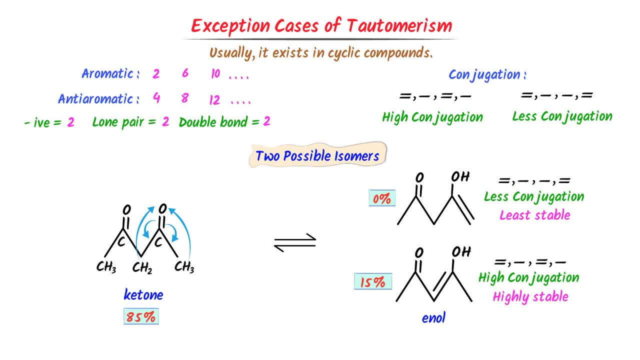 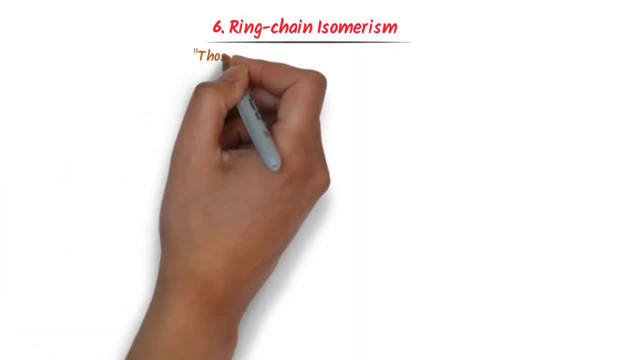 exception, cases of tautomerism. Now we will learn the last type of isomerism, which is ring chain isomerism. Well, those isomers having same molecular formula but different structures, like cyclic and open chain, Are called ring chain isomerism. 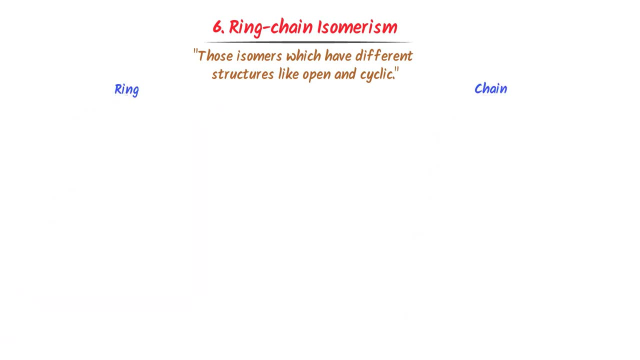 Here the word ring chain isomerism deeds the whole concept. The ring stands for cyclic isomer and the chain stands for open chain. So ring chain isomerisms are those which has one open chain compound and one cyclic compound. For example, consider propene. 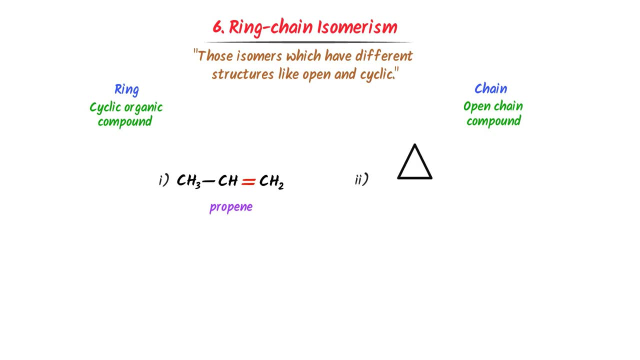 It is an open chain of propene. Now I convert it to cyclic structure, I get this structure. We know that this is acyclopropane. The molecular formula of the both compounds are the same, which is C3H6.. But they have different structure: open and cyclic. 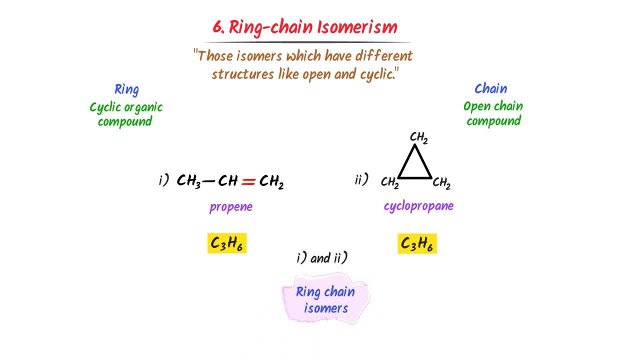 So they both are known as ring chain isomers. Secondly, consider hexene. I convert it to cyclic compound. I get this cyclic structure. It has no double bond. I call it cyclohexane. Here they both have the same molecular formula, which is C6H12.. 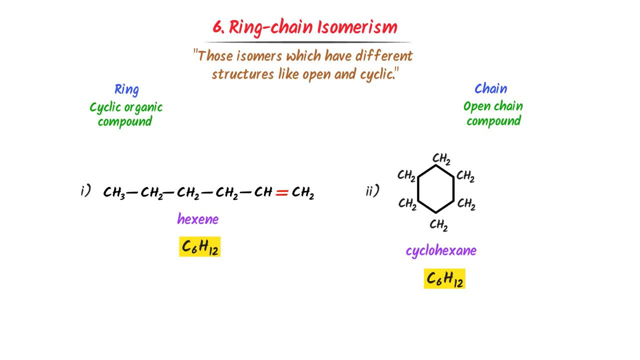 But they have different structures, like open chain and cyclic, So they both are ring chain isomers of each other. Thirdly, consider butene. Pause the video And try to make it a cyclic. So that's it. Now let's see how to make its ring chain isomers. 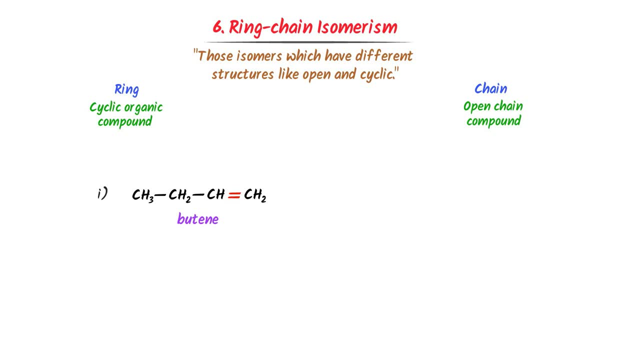 Well, it is super easy. Just convert it to cyclic structure having single bonds. I get this structure, which is known as cyclobutane. The molecular formula of the both compounds are the same, which is C4H10.. Just remember that ring chain isomers are those isomers which has one open chain and 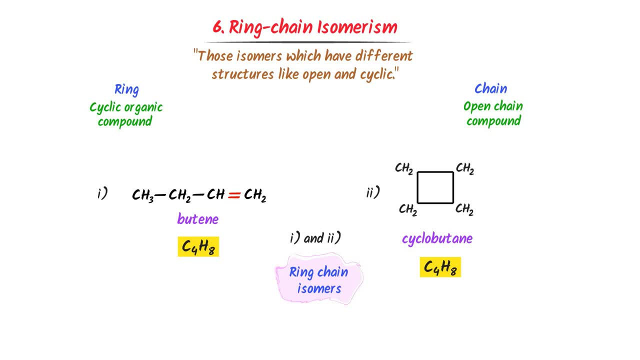 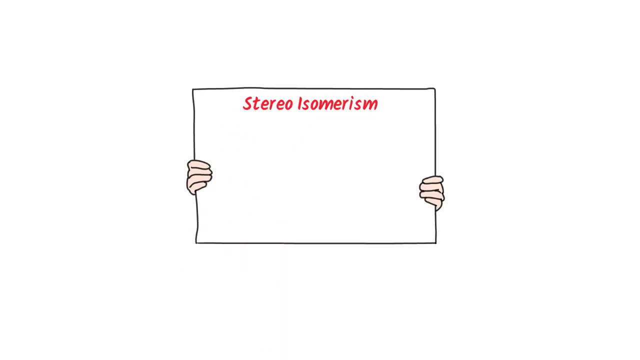 one cyclic. So we have learned the six different types of structural isomerism. Now we will learn stereo isomerism. Remember that in stereo isomerism, isomers have same molecular formula, same structural formula, but different arrangement of atoms in the space. 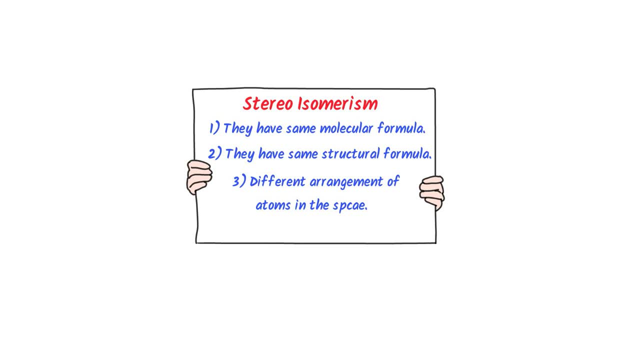 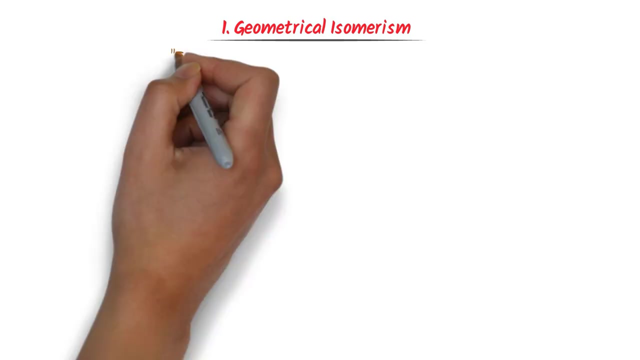 Hence, note it down, this important definition of stereo isomers. Now we will learn the first type of stereo isomerism. Now we will learn the first type of stereo isomerism, Which is geometrical isomerism. Remember that geometrical isomerism is also known as cis-trans isomerism. 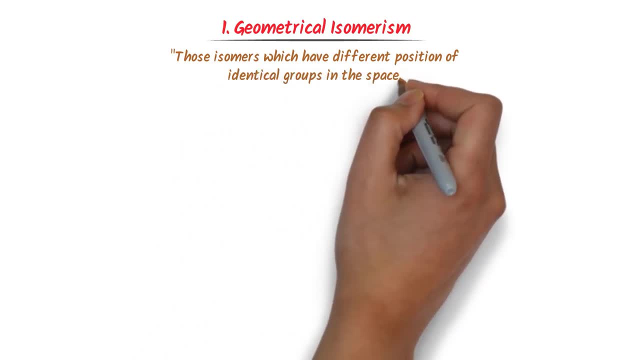 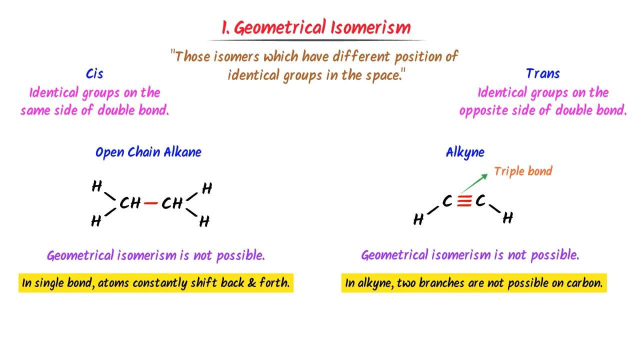 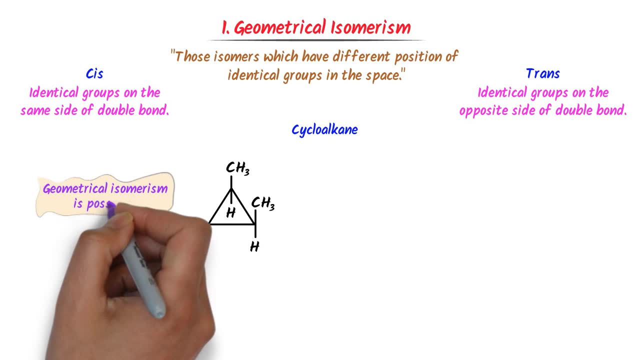 While trans means when two identical groups are present on the same side of double bond. Now consider this cycloalkane. The question is: is geometrical isomerism possible in cycloalkane? Well, the answer is yes, For instance in this compound. I write up and down: 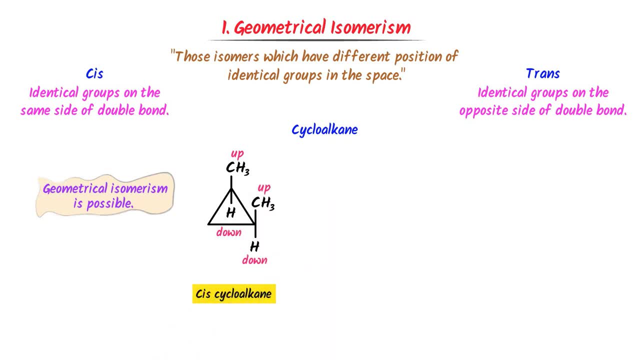 Up and down. So this is a cis-cycloalkane. So this is a cis-cycloalkane. Now I just interchange the up and down position of the CH3 group. Now, I just interchange the up and down position of the CH3 group. 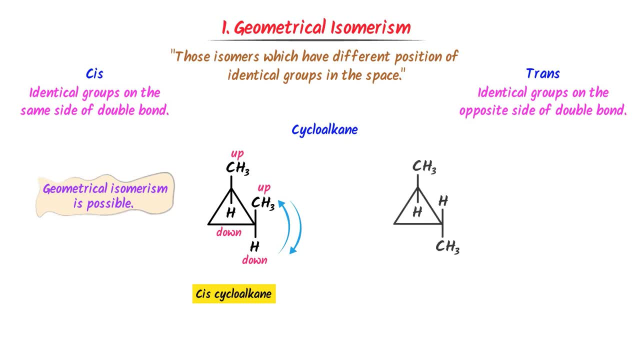 and hydrogen hydrogen group. I get this compound. Here the alkyl group CH3 is up and here the alkyl group is down. Hence it is a trans cycloalkane. Just remember that geometrical isomerism is possible in cycloalkane. 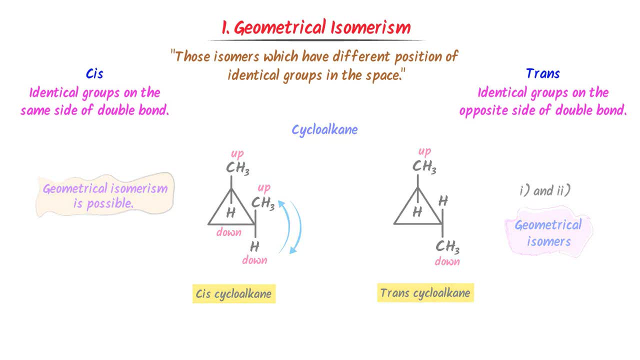 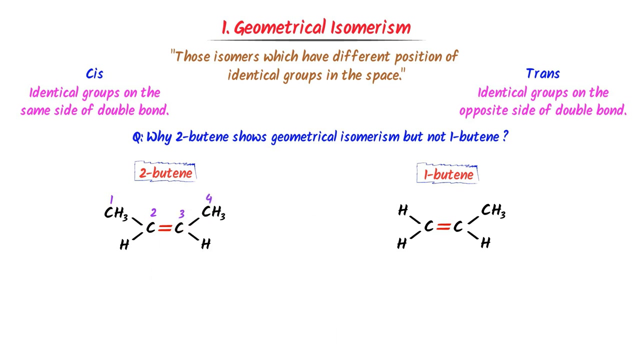 Let me teach you one another important question: Why two butene shows geometrical isomerism, but not one butene? Well, consider two butene and one butene. Now I write 1,, 2,, 3, 4.. The double bond. 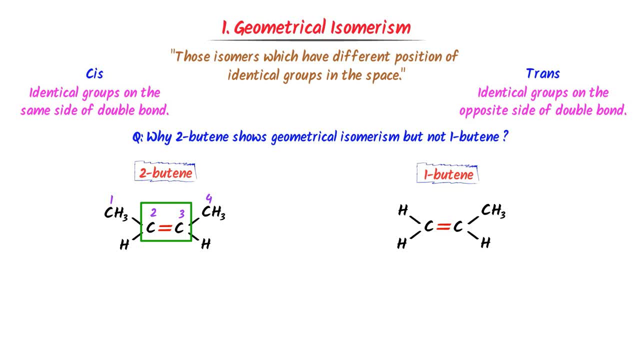 is present at the second position. We call it two butene. On the second and third carbon, two different groups are attached to the same carbon atom. Hence geometrical isomerism is possible in it, While in this compound I write 1,, 2,, 3.. 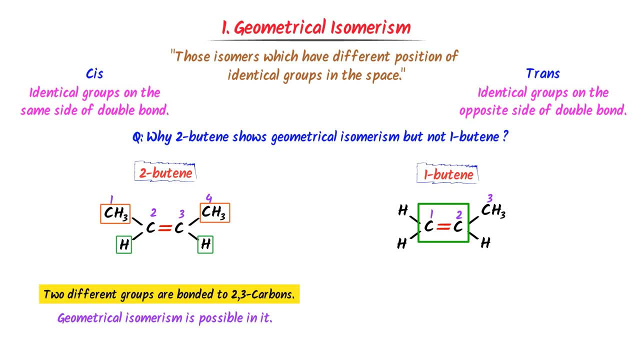 The double bond is present at the first position. I write 1 butene Here. on the second carbon there is alkyl group and hydrogen group. So it is all right. But here at first carbon, the two same groups- hydrogen- are attached to the first carbon. We have already learned that. 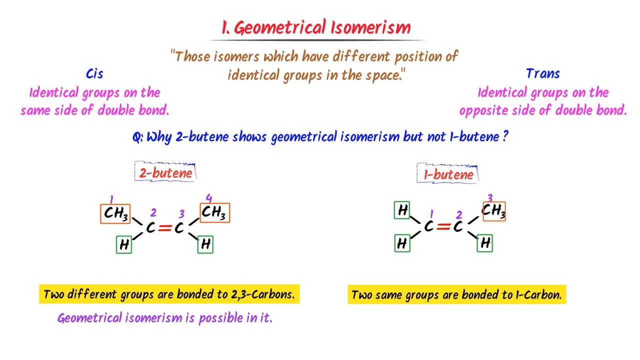 if identical groups are attached to the same carbon, geometrical isomerism is not possible. Therefore, geometrical isomerism is not possible in one butene, but it is possible in two butene. Hence, note it down, this important question. 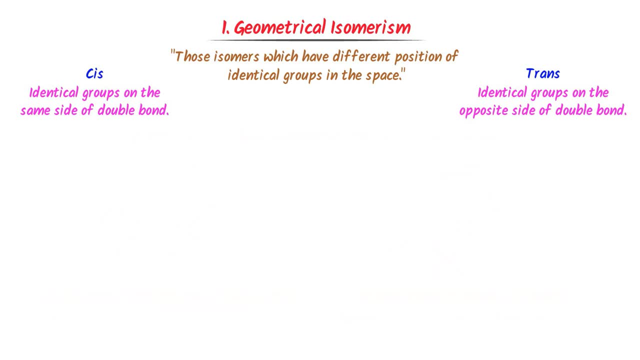 The final concept of geometrical isomerism is Z and E form. Consider this organic compound. Here, the four groups bonded to two carbons are different. In such cases, we decide on the basis of atomic size. In this case, we decide on the basis of atomic size. Here, the four groups bonded to two carbons are different. In such cases, we decide on the basis of atomic size. 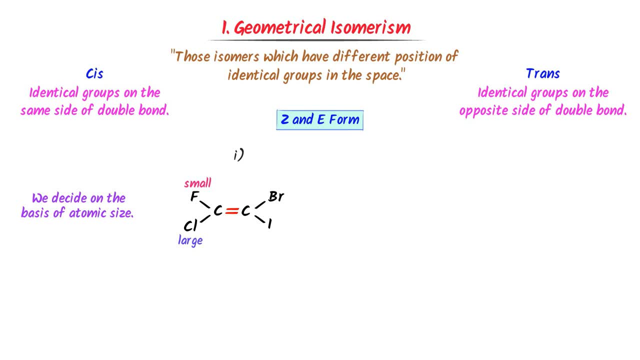 Here the four groups bonded to two carbons are different. In such cases we decide on the basis of atomic size. Fluorine has the smaller size than chlorine, while bromine has the smaller size than iodine. Now, the smaller size groups are at the same side of double bond, Hence it is a cis form. 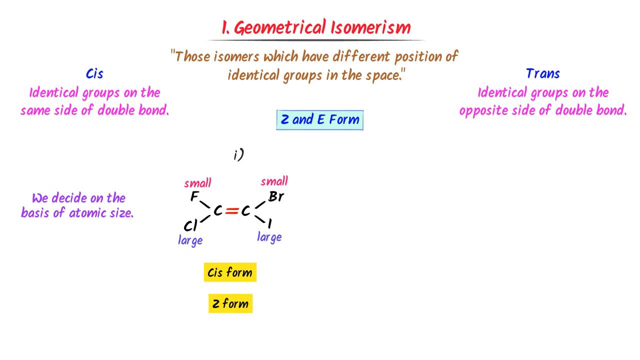 or we call it Z form. Now, as usual, I interchange the smaller size and larger size groups of bromine and iodine. I get this compound Here. fluorine has smaller size than chlorine, while iodine has a larger size than bromine. The smaller size groups. 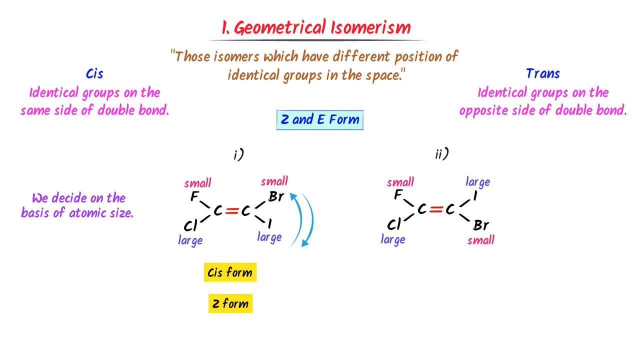 like fluorine and bromine, are at the opposite side of the double bond, so we call it transform or we call it E form. thus, these are the two geometrical isomers of each other and we call it Z form and E form, hence, noted down this. 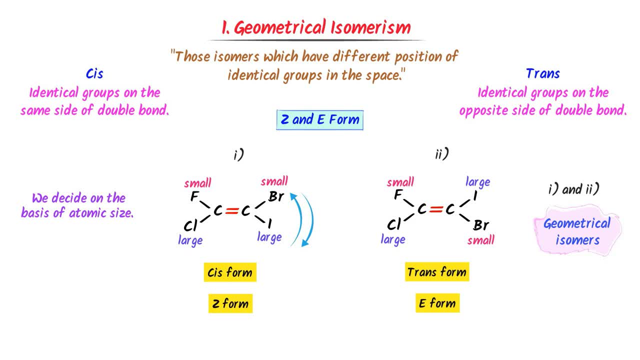 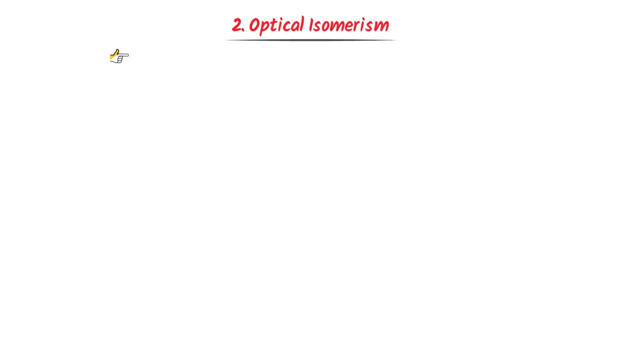 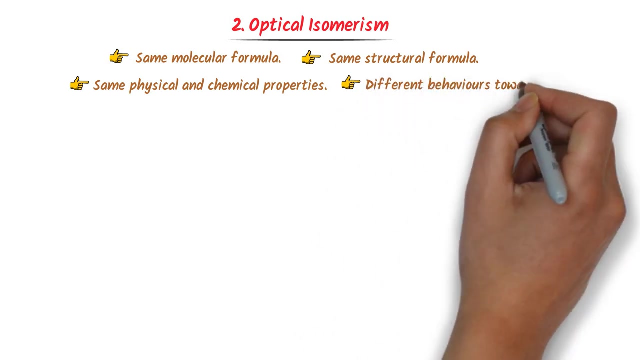 important concept. finally, let me teach you the most difficult isomerism, which is optical isomerism. optical isomers have these four properties. they have same chemical formula, they have same molecular formula, they have same chemical and physical properties. the only difference between them is that they have different behaviors towards light. now I will teach you only two. 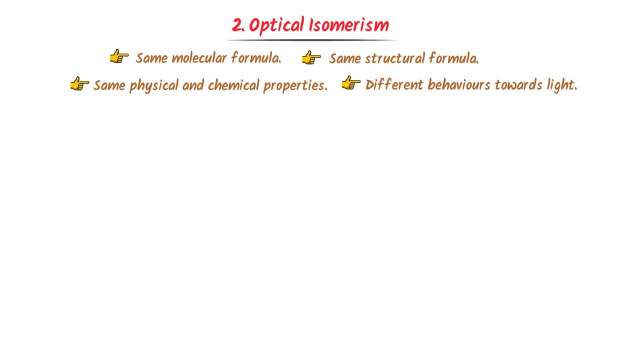 conditions for optical isomerism, and it will help you to master this concept. the first one is optically active substance and the second one is asymmetrical carbon. for example, consider this compound. if this compound is optically active and it has a symmetrical carbon, then optical isomerism is possible in. 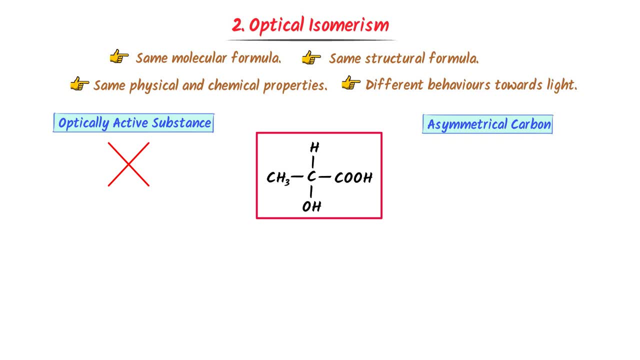 it. if it is not optically active or it has no asymmetrical carbon, then it will not show optical isomerism. now, what is optically active? isomerism and isometrism? dimethyl isomerism is not edible to the active compounds. Well, to learn it, we have to learn polarized light, polarimeter optically. 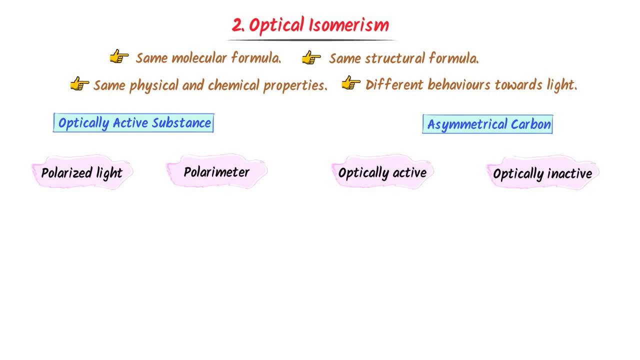 active compounds and optically inactive compounds. Now the light in one direction is called polarized light, For example. this light is going in one direction, It is known as polarized light, While the light produced by the bulb is called unpolarized light, because it spreads in all. 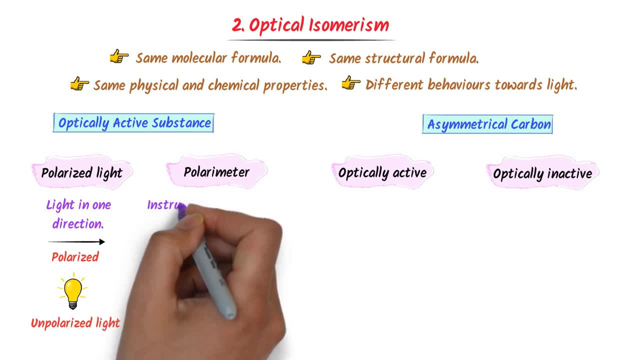 direction. Secondly, polarimeter is an instrument which is used to measure the polarization of light and optical activity of a compound. Thirdly, the substances which can easily rotate the polarized light are called optically active substances. For example, consider glucose. 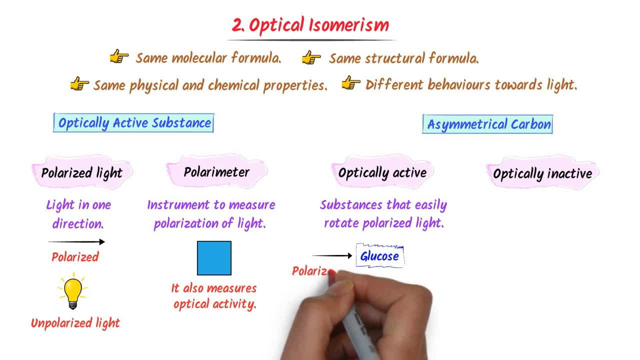 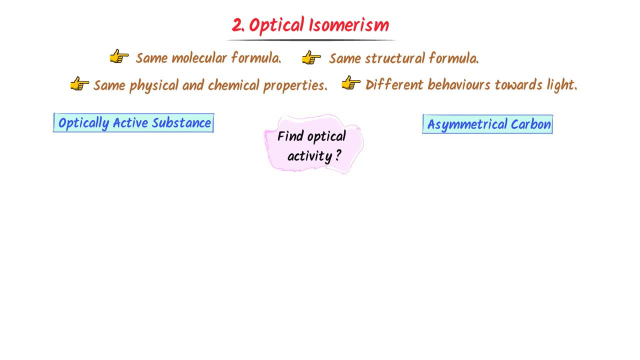 Well, we use nickel prism and polarimeter to find the optical activity of a compound. For example, we take a light source. It produces light in all directions. Here it is unpolarized light. I place nickel prism in front of it. 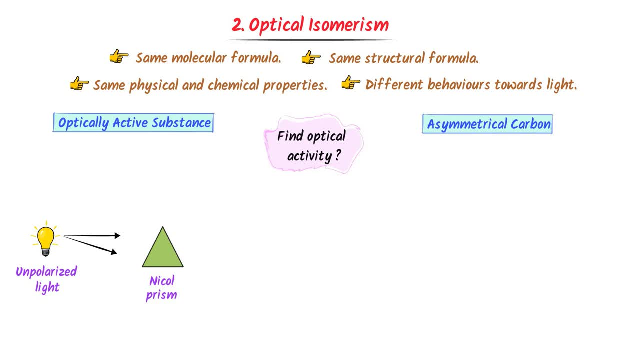 Now the nickel prism. simply convert the unpolarized light to polarized light. Secondly, I make a solution of a compound and place it in the polarimeter. Now there are three possible outcomes. If the light is rotated in the left direction, 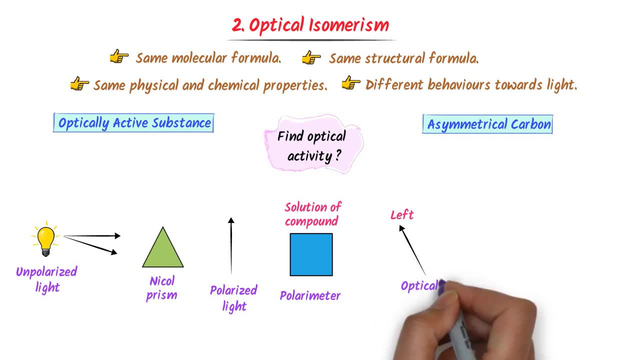 or anticlockwise direction. the substance is optically active and we call it Leo-rotatory compound. We represent it by negative sign. If the light is rotated in right direction or clockwise direction, the substance is optically active and we call it. 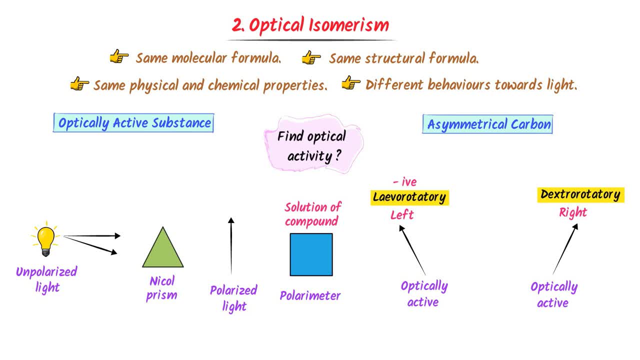 dextrorotatory compound, We represent it by positive sign. Lastly, if the light is not rotated in the left or in the right direction, it means that compound is optically inactive. Thus, remember that if a compound rotates light in left direction, 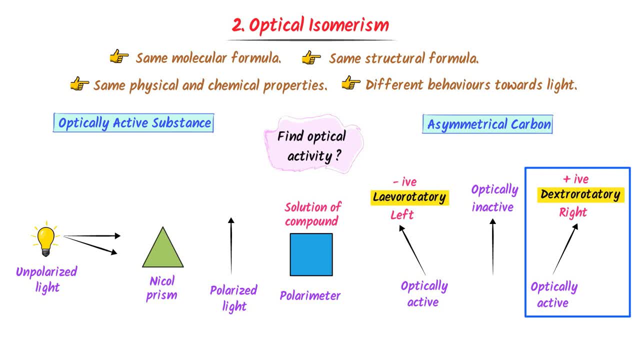 it is Leo-rotatory. If a compound rotates lights in right direction, it is dextrorotatory. Now we will learn the second condition for optical isomerism, which is asymmetrical carbon. Firstly, we will learn asymmetrical compounds, For example. consider these compounds Here. 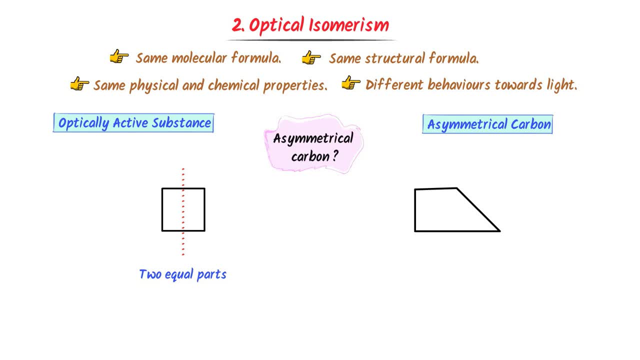 we can easily divide this compound into two equal parts, So it is symmetrical compound, While we cannot divide this substance into two equal parts because this part is different from this part, So it is asymmetrical compound. Now consider this compound. Here, four different groups are. 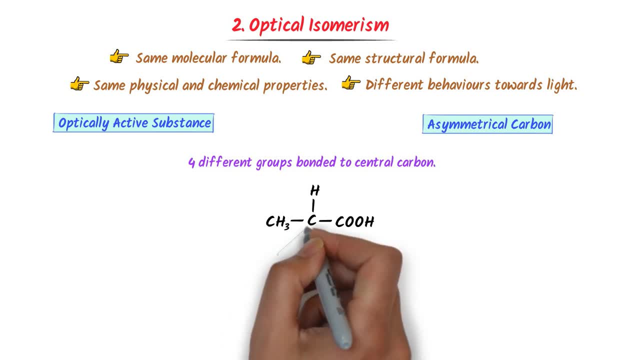 attached to the carbon. We call this carbon as asymmetrical carbon because if we divide this compound at this carbon, we get two different parts. So it is asymmetrical carbon. To summarize, to summarize this whole concept, we have learned that for optical isomerism we need an optically 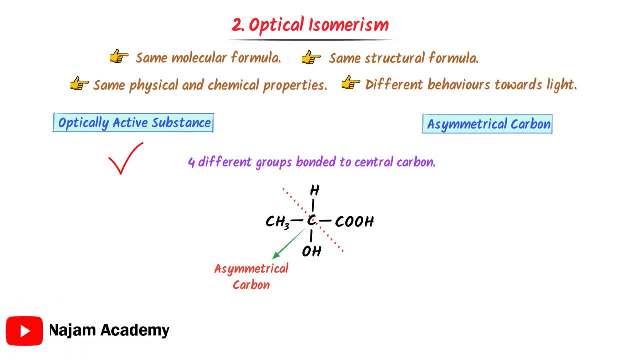 We need optically active compounds. Secondly, the compound must have one asymmetrical carbon. Now we will learn the optical isomers of lactic acid. Well, consider the lactic acid. I write 1,, 2, 3.. Its IUPAC name is 2-hydroxypropanoic acid. 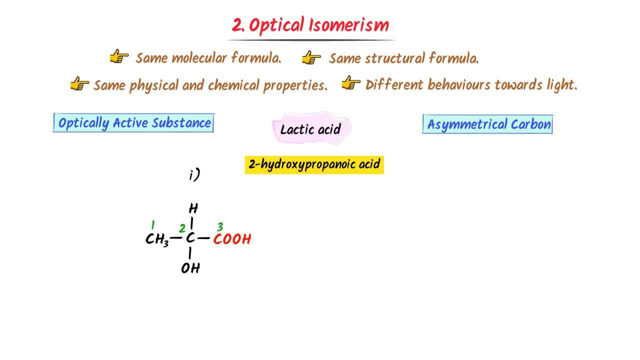 I look for the conditions. It has asymmetrical carbon, So it is optically active compound. Now I place a mirror in front of it. We know that in the mirror the right side becomes left and the left side becomes right. I get this compound. 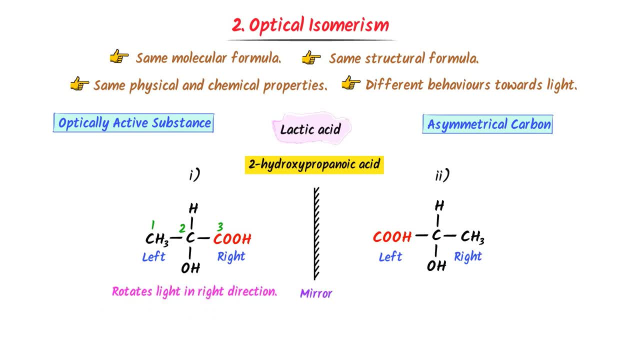 Now listen carefully. It rotates polarized light towards right direction. We call it dextrorotatory And we represent it by positive sign. Secondly, it rotates polarized And in the case of polarized light towards left, we call it leurotatory. 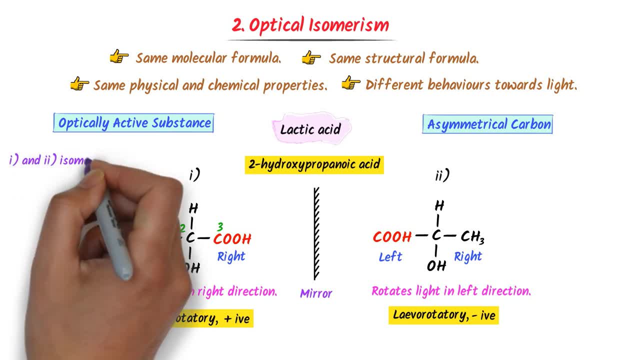 And we represent it by negative sign. This first and second isomers are called enantiomers. Enantiomers are those isomers which are mirror images of each other. Let me repeat it: Enantiomers are those isomers which are mirror images of each other. 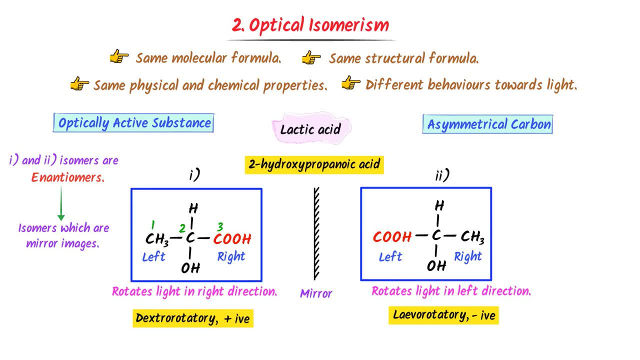 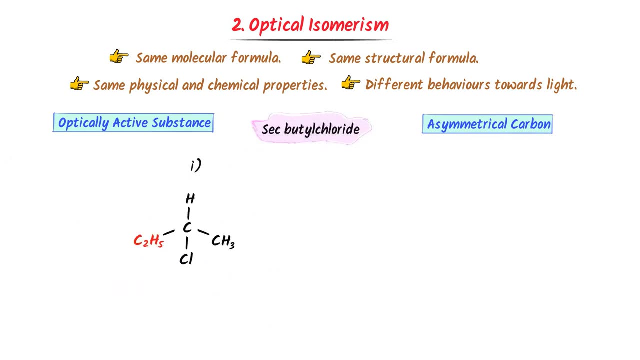 Thus remember that. And the second isomers are called enantiomers because they both are mirror images of each other. So these are the two optical isomers of lactic acid. Now consider secondary butyl chloride and form its optical isomers. 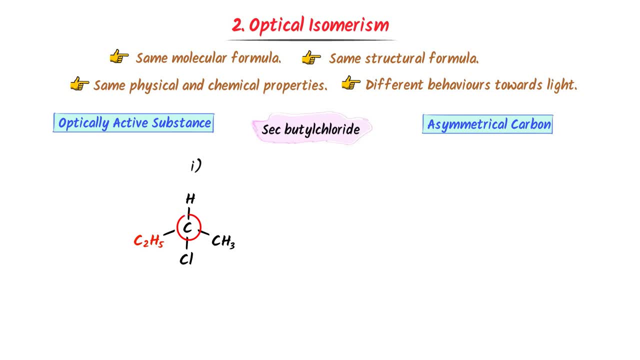 Well, we can see that this carbon is asymmetric because all the four carbon attached to this carbon are different, So it is optically active compound. Now I place mirror here. As a result, I get this compound. This CH3 is here and this C2H5 is here. 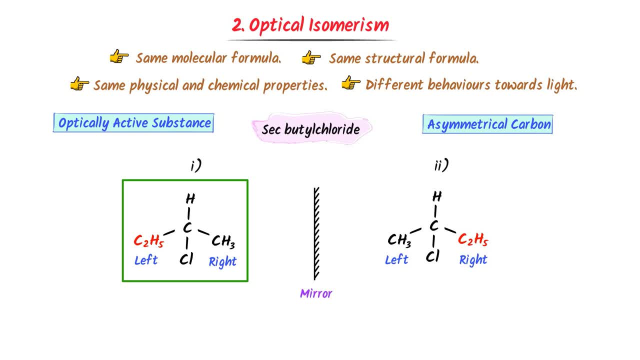 Now it depends on you to call this compound negative or positive. Let, this is negative. We call it leu-rotatory isomers. This is positive. We call it dextro-rotatory. We know that these both are enantiomers of each other, because they are mirror images of each other. 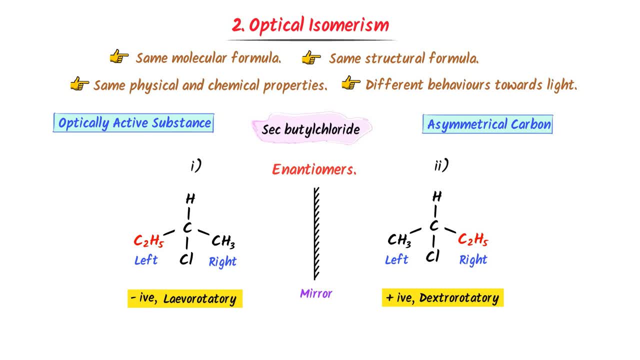 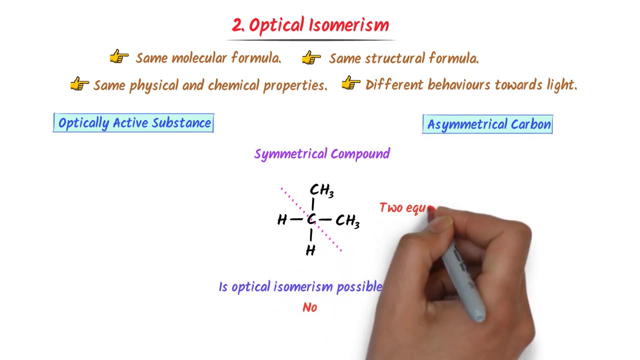 So these are the two optical isomers of this compound. Now consider this organic compound. Is optical isomerism possible in it? The answer is no. This compound is symmetrical. If I cut this compound from here, I get equal parts on both sides. 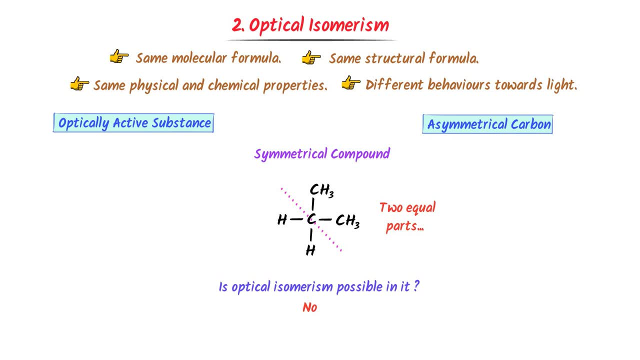 Hence it does not show optical isomerism. Finally, consider optical isomerism in tartaric acid. Well, consider its structure. Remember that hydroxyl groups and OH group are present at opposite side. This compound is asymmetric. 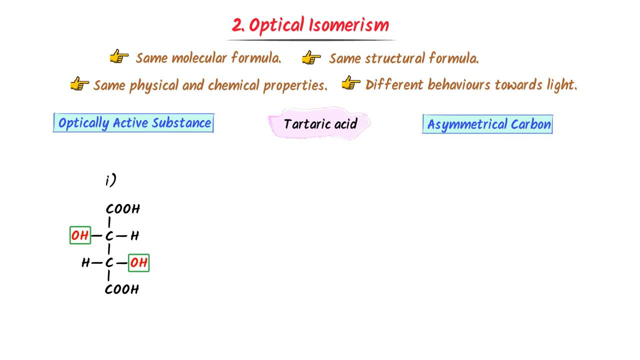 Hence optical isomerism is possible in it. I write 1,, 2,, 3,, 4.. It's second and third position, Hydroxyl group. Hydroxyl groups are present. I write 2, 3-dihydroxybutane. 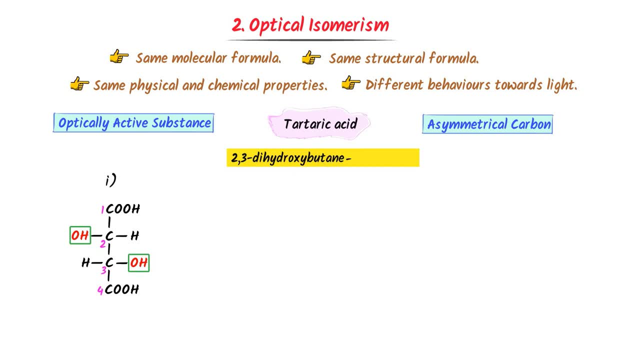 While at first and fourth position carboxylic acid groups are present, I write 1, 4-dioic acid, So its IUPAC name is 2, 3-dihydroxybutane-1, 4-dioic acid. 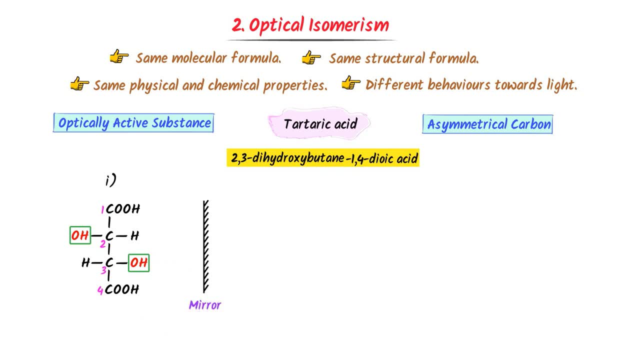 Now, as usual, I place mirror in front of this compound. I get this compound. This OH shifts here and this OH shifts here. Let we call this dextrorotatory tartaric acid And we represent it by positive sign. 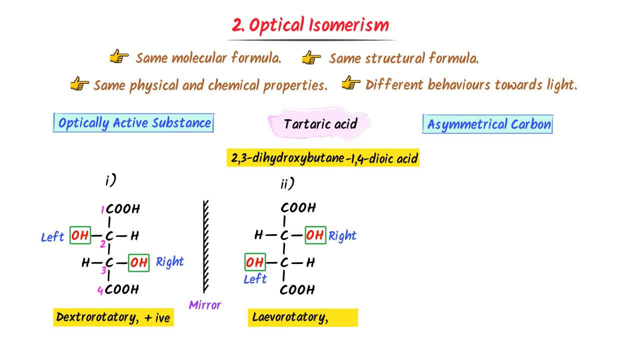 We call this leurotatory tartaric acid And we represent it by negative sign. These both isomers are enantiomers of each other, because they are both mirror images of each other. The third isomer of tartaric acid is: 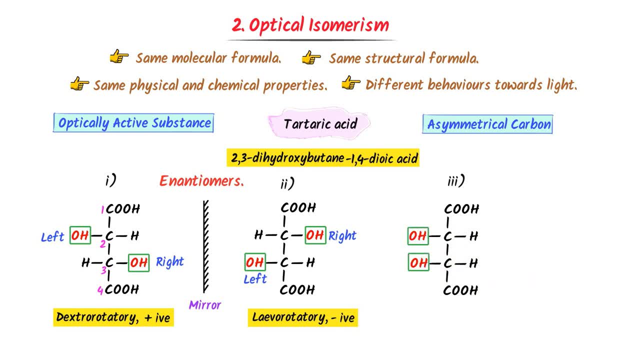 this one. Here the OH groups are present at the same site. We can see that this carbon is asymmetric because different groups are attached to it And similarly, this carbon is also asymmetric because different groups are attached to this carbon. But wait a minute. 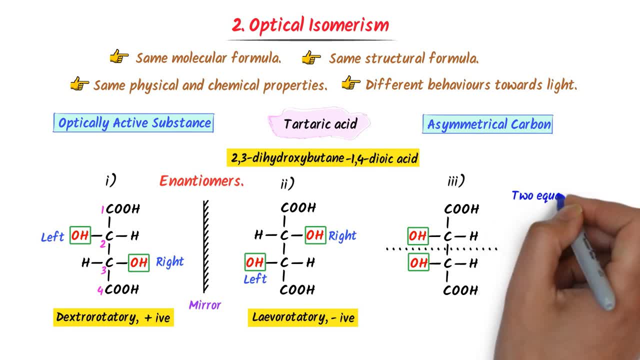 If I draw a symmetrical line here, I get two equal parts. Hence this compound is symmetrical compound And optical isomerism is not possible in it. So we say that it is also optically inactive compound. We call it meso-tartaric acid. 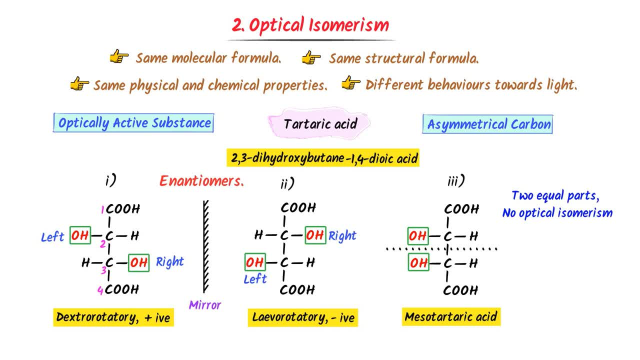 Thus optical isomerism is not possible in it. Here you must learn the concept of deisteromers. Those isomers which are not mirror images of each other are called deisteromers. For example first isomer and third isomers are not mirror images of each other.